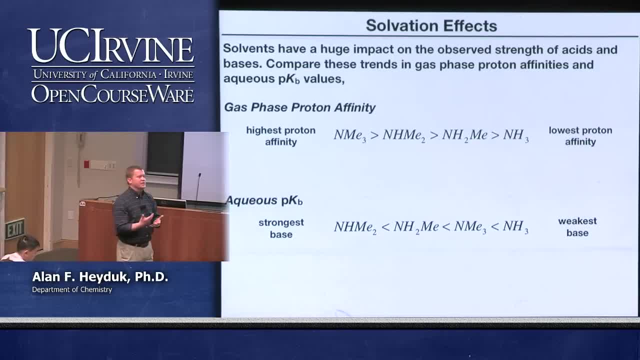 a fantastic hydrogen bonding solvent and you can form these intermolecular forces between water molecules and the proton, The protonated dimethylamine that helps stabilize that cation. So the dimethylamonium is very well stabilized in water because it can form a hydrogen bonding network, whereas trimethylamine. 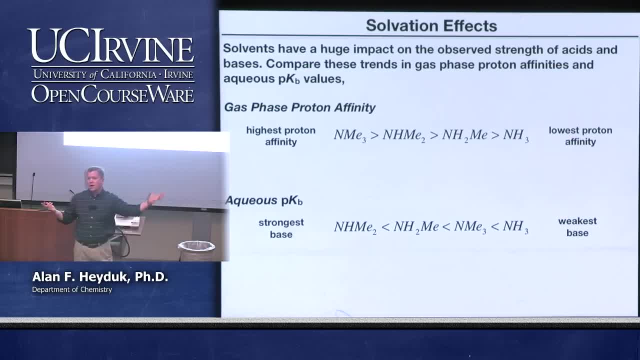 can't form as many hydrogen bonds. Methyl groups can't hydrogen bond, so it's not as well stabilized in water. Every time you see this, these kind of relationships, acid base, you see, these orderings, all we're all we're talking about are equilibrium, okay, We're talking about which one? which product? 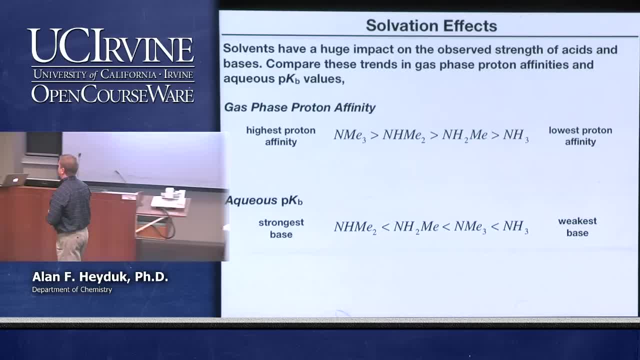 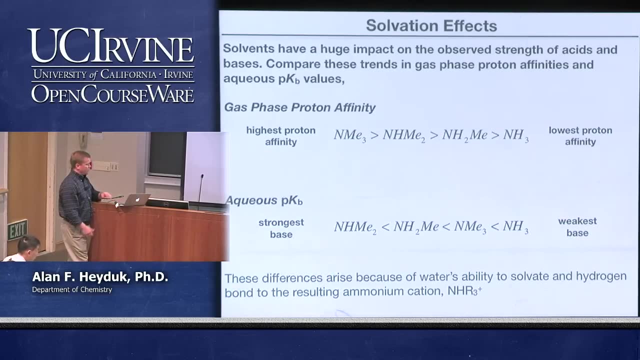 is most stable and in this case, the protonated form of dimethylamine or the dimethylamonium cation is more stabilized by water than the trimethylamonium or the protonated form of trimethylamine. Okay, we also saw this table last time that lists the pH of hydrogen. So 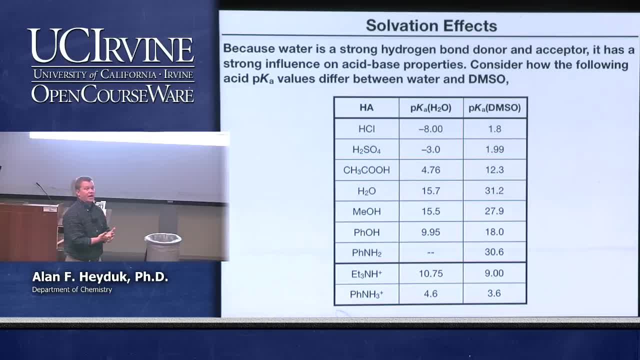 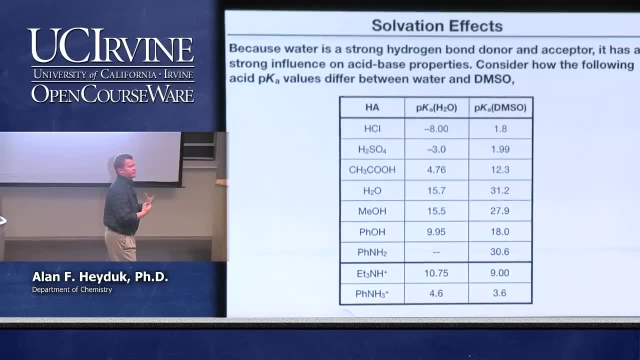 PKA of various acids in water and in an organic solvent, DMSO, dimethyl sulfoxide. So again, we all know that water is fantastic. It can stabilize cations, It can stabilize anions, It can be a hydrogen bond donor. 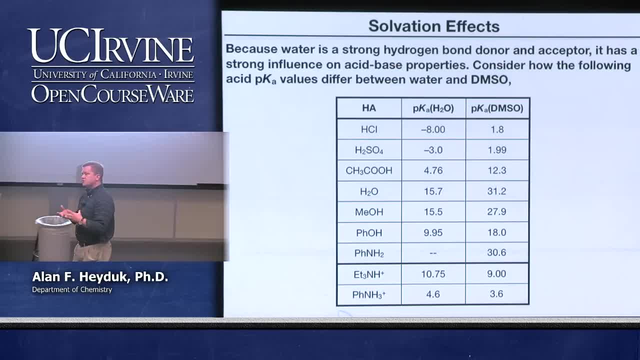 It can be a hydrogen bond acceptor. DMSO is for an organic solvent. it's great with cations and anions. Okay, It's got an oxygen on it that has a strong delta minus, So it can help stabilize cations. 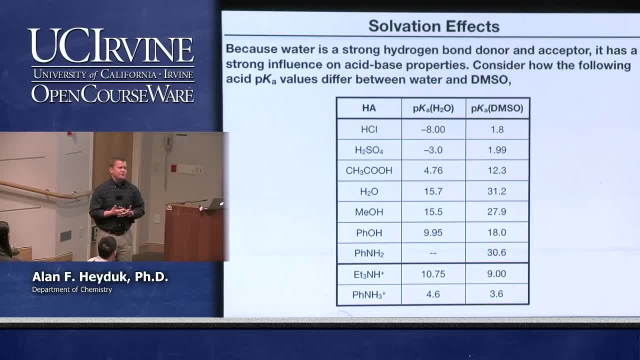 But what it doesn't have is a region of the molecule that's delta plus. I mean it does, It's the sulfur, but it's buried, Okay, It's not accessible, And so it's not really great at stabilizing anions. 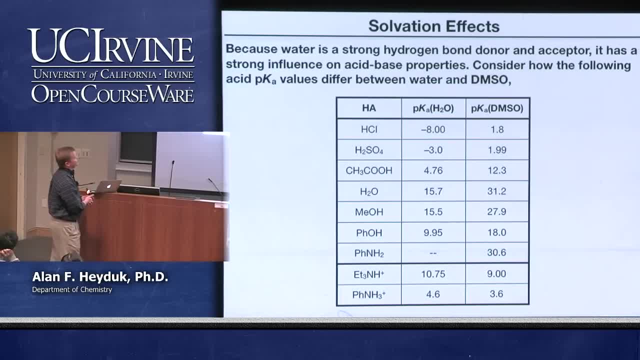 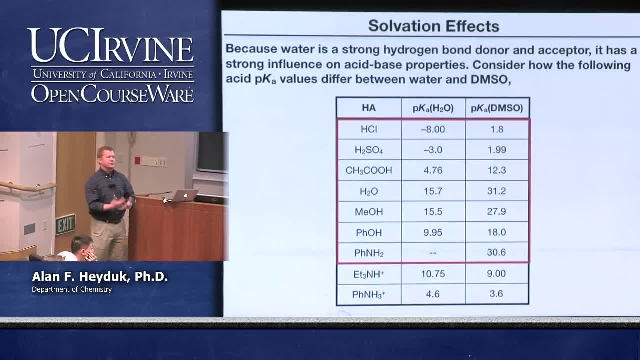 which are all the neutral acids. Okay, These are things that are neutral molecules that will lose a proton to give up the positively charged proton and the negatively charged A minus whatever the corresponding or the conjugate base is. All of these acids are significantly stronger in water. 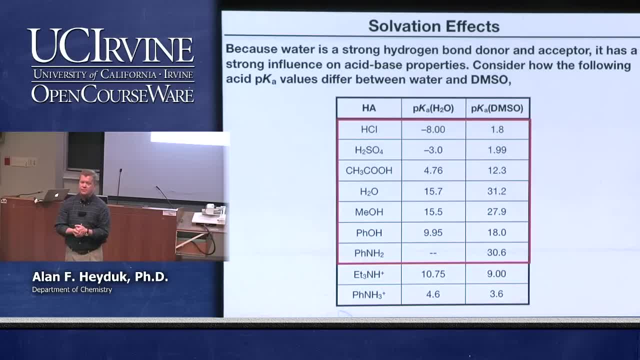 than they are in DMSO. And this strictly comes about because water can stabilize both the proton that comes off and the anion, the anionic base, that comes out. Okay, In DMSO that anionic base isn't stabilized very well. 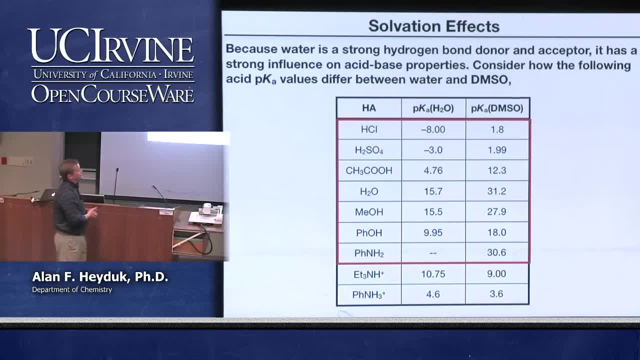 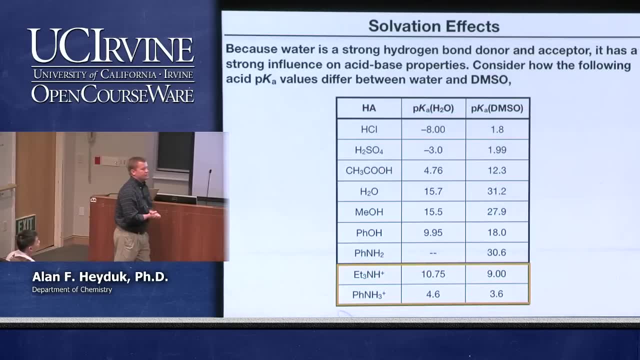 So, correspondingly, all of these neutral acids are weaker acids in DMSO than they are in water. Now, what we see at the bottom are cationic acids. Okay, You'll recognize these as the conjugate acid of many of our favorite bases. 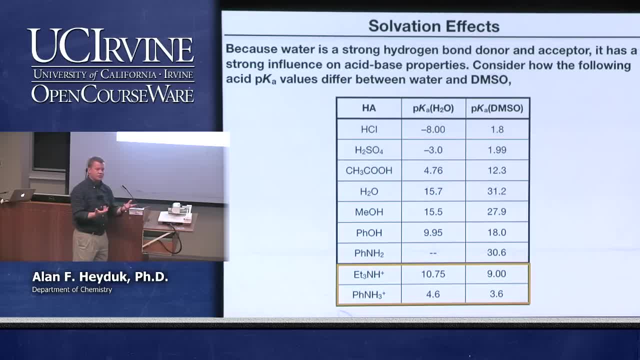 So if we have the triethylammonium, which is the triethylammonium, the triethylammonium acid- okay, it's the conjugate acid of triethylamine- you'll notice that it's a stronger acid in DMSO. 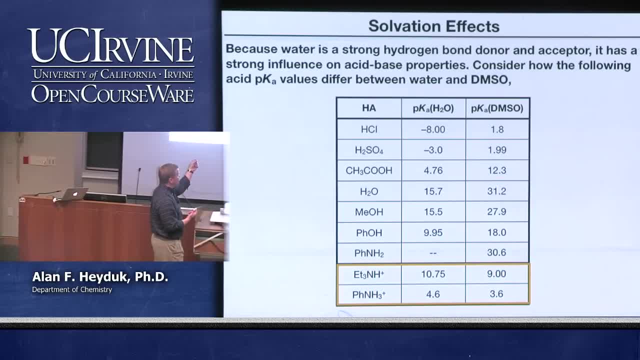 Why? Well, because in DMSO, if you think about what happens with this acid, you dissolve it, a proton pops off and you're left with a neutral base. The DMSO is better with the neutral base than the water is. 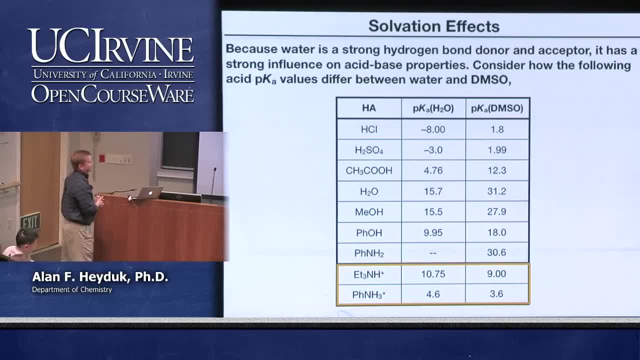 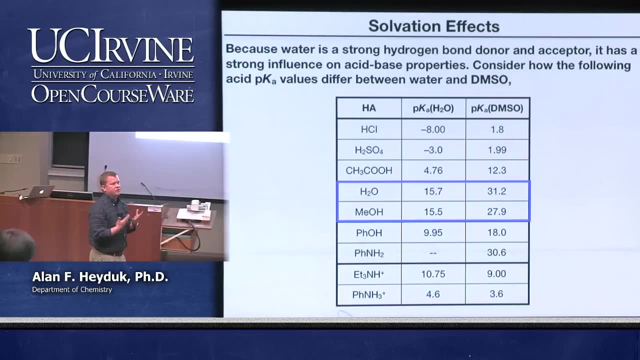 Okay And so. So, therefore, these charged acids, these cationic acids, are typically stronger in DMSO than they are in water. This is one of these things. It's kind of a recurring theme in chemistry. Everything I ever needed to know. 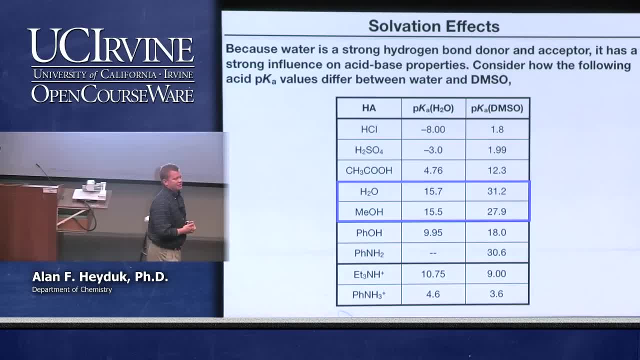 I learned in freshman chemistry. You may have heard that you learned it in kindergarten. That's not really true. I was still smearing paint with my hands in kindergarten, so But really like all of this. all of this is just the basic intermolecular forces. 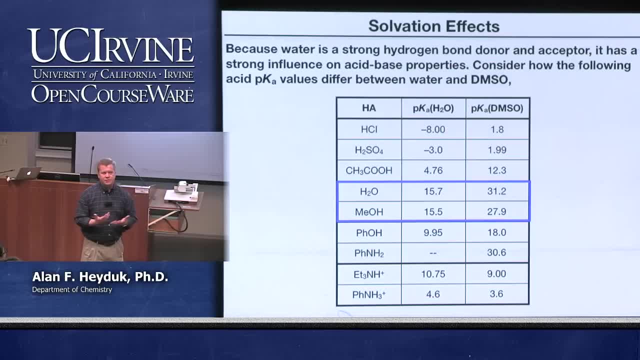 delta G's free energies equilibria that we learned in freshman chemistry. We're just applying it in more and more sophisticated ways, So you should always, if you're ever confused, make sure you can write out the equilibrium and understand what the reactants. 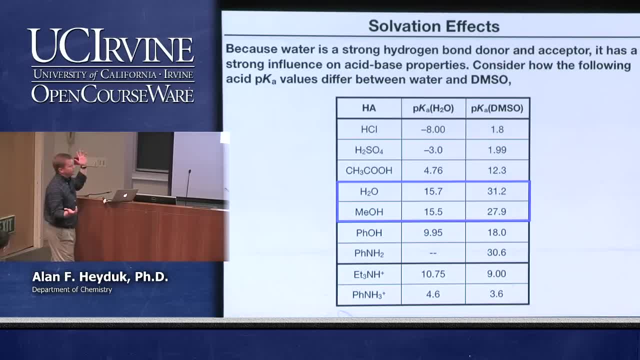 and what the products are, and that'll help you understand what these PKA values mean. Water and methanol- I highlight this one because everybody thinks that water is a stronger acid than methanol. is right. We all say, oh, water has a PKA of 14.. 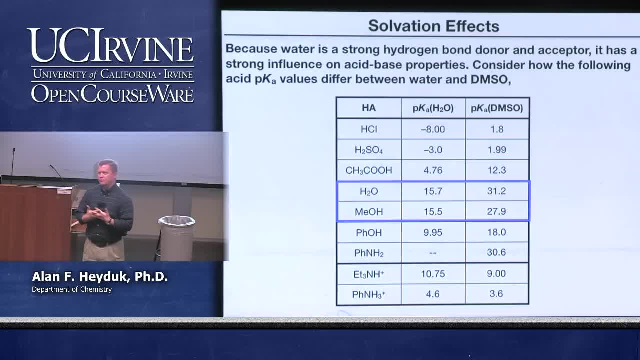 That doesn't take into account that water. when you're measuring the acidity of water in water it's 55 molar instead of 1 molar. So when you take into account the concentration of water, it's actually a weaker acid than methanol, even in water. 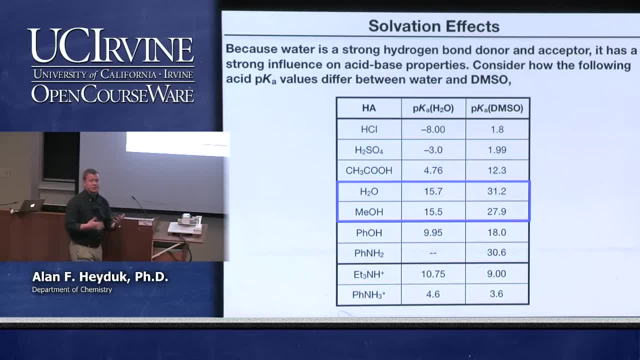 We can definitely see that when we switch to water, We switch over to DMSO, where they're measured under similar conditions, and water is about four orders of magnitude, three orders of magnitude, three and a half, whatever- weaker than methanol. 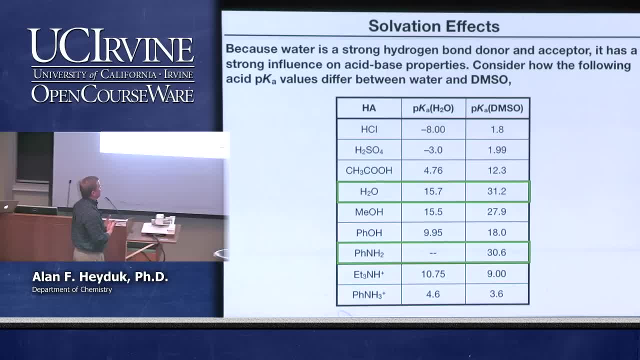 We can even see that in when we compare water to something like aniline. Most of us don't think of aniline as an acid. We think of it as a base right. It's a primary acid. Right, Right, Right. 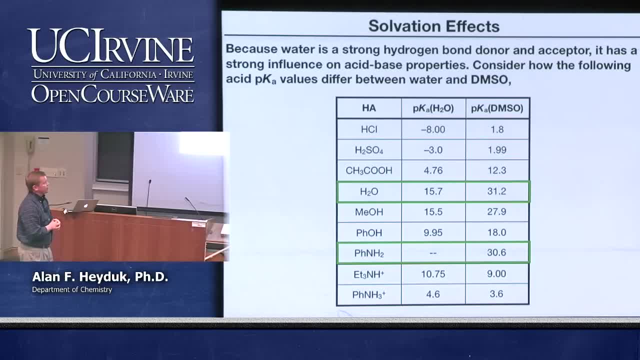 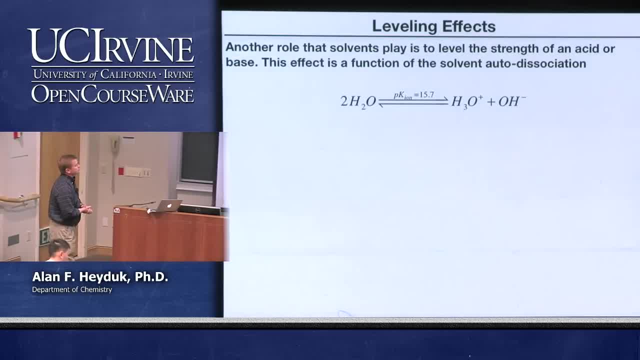 Okay, Fun with numbers. Okay. the other big effect that solvent has on acid activity, if you will, is what we call the leveling effect And, simply stated, the strongest acid you can have in water solution is the hydronium ion H3O plus. 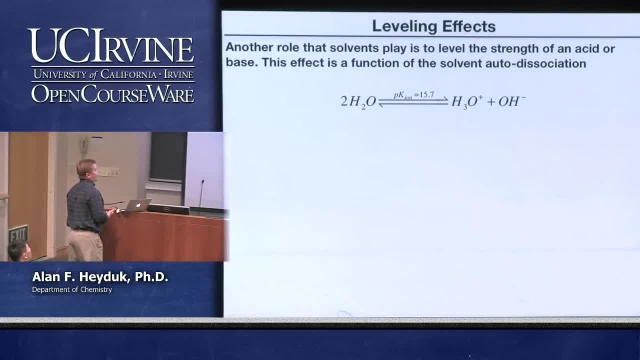 Okay, It's. any time you dissolve a stronger acid in water, the proton transfers to a water molecule, you make H3O plus and you're done. And so again, here's the dissociation of water to give H3O plus and OH minus. 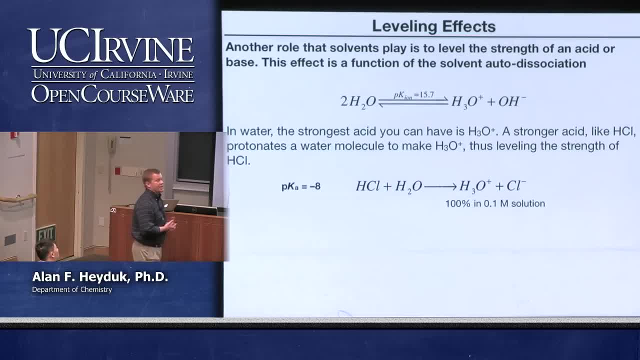 And so we can ask what happens if we take HCl, which is a very strong acid, We can estimate the pKa to be minus 8.. If we dissolve it in water, even in very dilute solutions or marginally dilute 0.1 molar, it completely dissociates. 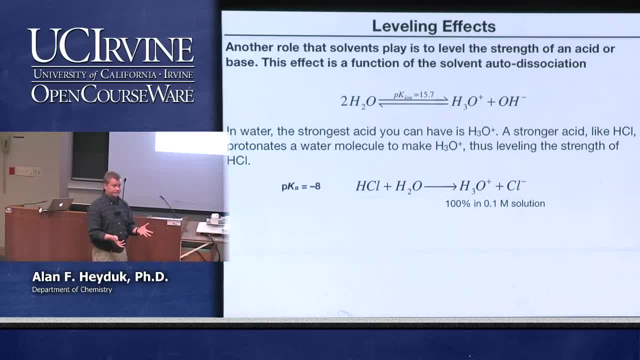 We get hydronium cations and chloride anions. So again, the strongest acid in solution is the H3O plus cation. If we were to use nitric acid- also a strong acid, dissolve it in water, make a 0.1 molar solution. 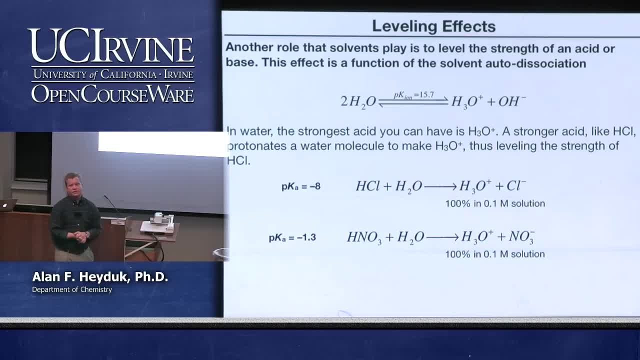 we would get 100 percent dissociation to H3O plus and the nitrate anion, the conjugate base of nitric acid. Okay, These are stronger acids than water. As you're dissolving it, they get they completely dissociate. 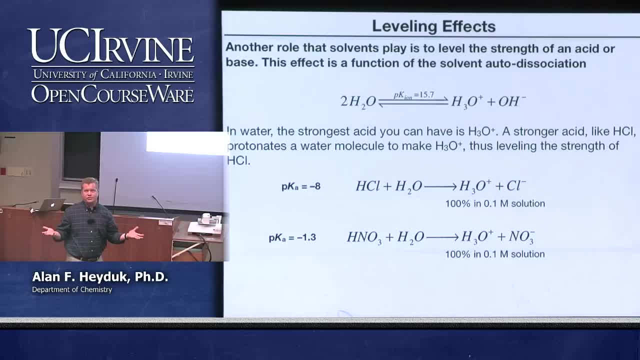 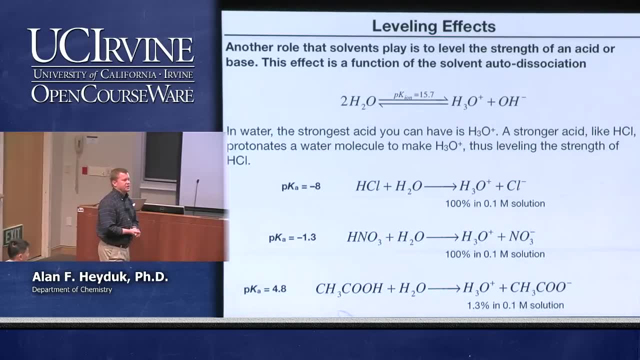 and you're still left with the hydronium ion as the strongest acid around. Well, what happens then when we use a weaker acid Like, let's see, Acetic acid vinegar? Well, it turns out that when you dissolve acetic acid, 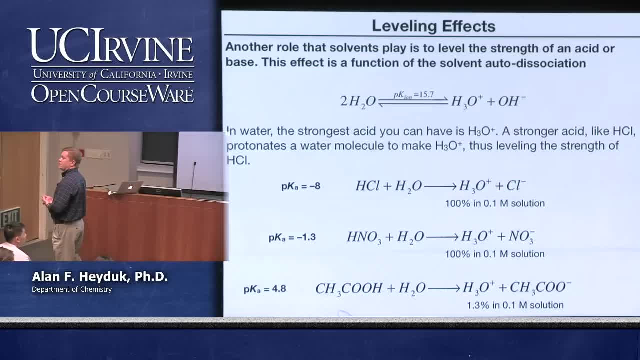 in water. you do make the hydronium ion, But you don't make as much. So again, a 0.1 molar solution of acetic acid in water is only 1.3 percent hydronium ion and the rest 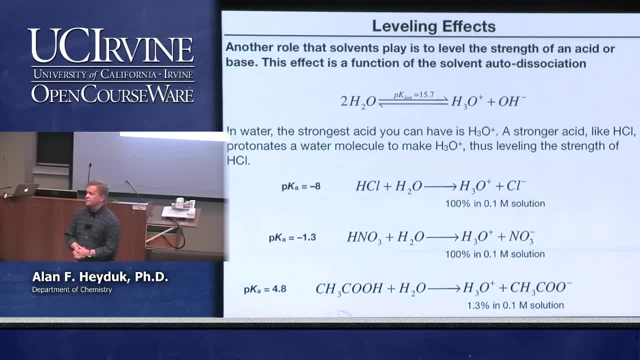 right. Professor Haddox made his first mistake. These should all be equilibrium arrows, And in this last reaction the equilibrium should lie far to the left. Okay, If only 1.3 percent is hydronium ion plus acetate. 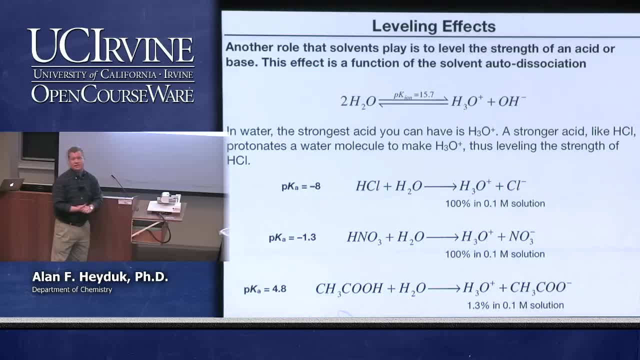 anion, that means 98.7 percent is still acetic acid and water. Okay, So the strongest acid you'll ever get in a solvent is the protonated version of the solvent itself. It's what we call the leveling effect, And what it gives rise to is windows of acidity. 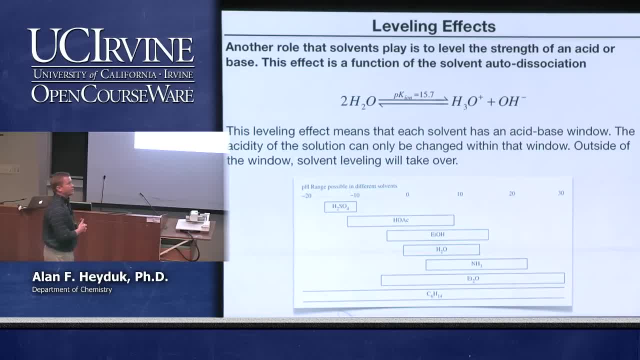 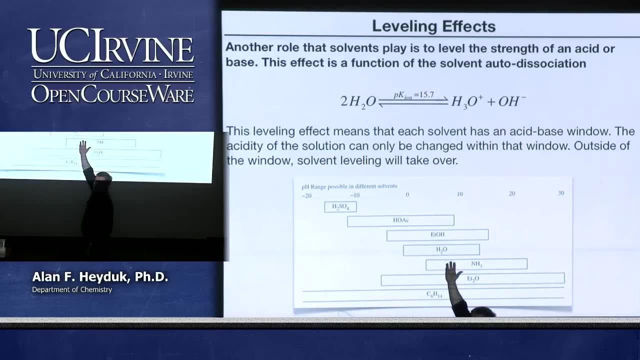 or basicity for each solvent. Okay, You're only going to be able to access a range of pHs in each solvent. So right here in the middle, you see that water has a relatively narrow range. Okay, Because of the formation of the autoionization. 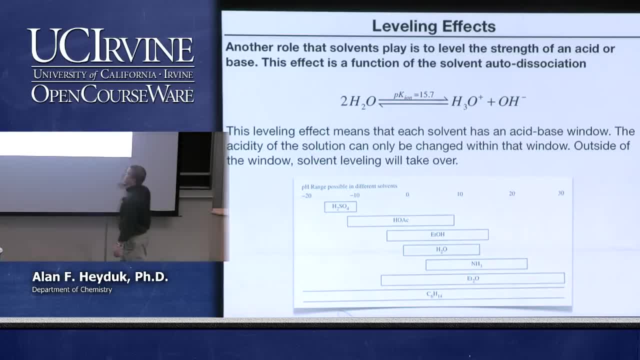 you get hydronium ions and you get hydroxide anions And so roughly you can go from about zero to 15 for water solutions. Ethanol is a little bit broader Acetic acid. we don't usually think of acetic acid. 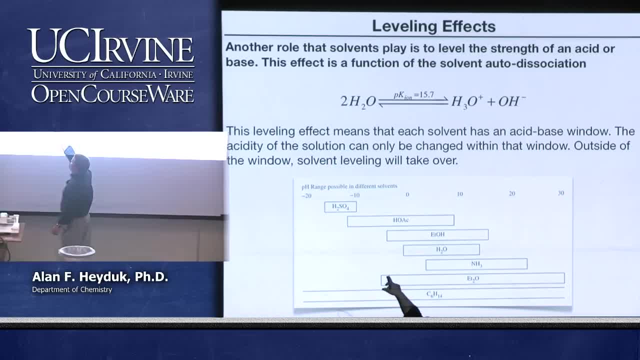 as a solvent, but you can use it as a solvent. There you can get to pretty acidic pHs minus 11, but you can only get up to a pH of about nine, right, Because again, acetic acid has its own dissociation. 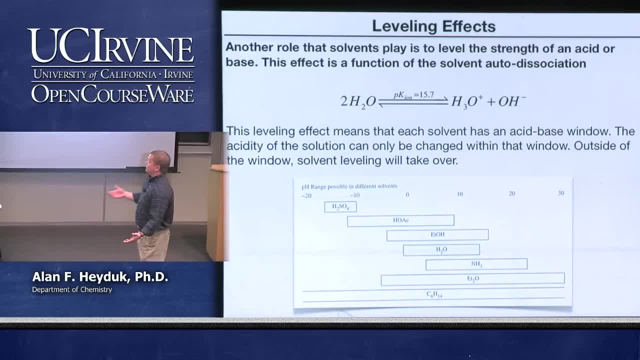 to protons and acetate, And if you get more basic than a pH of nine, well, you're just going to level out to acetate. I wouldn't recommend using sulfuric acid as a solvent, but it can be done. This one's kind of interesting. 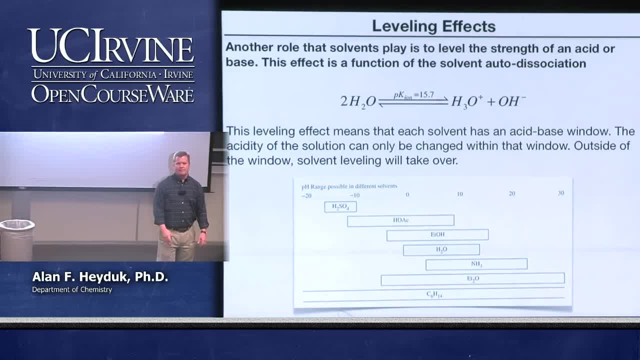 Hexanes, You'll notice it's the only one that doesn't have boundaries on this chart. Who wants to take a stab at why It doesn't get protonated or deprotonated? Yeah, When in organic chemistry did you learn about- you know, the dissociation. 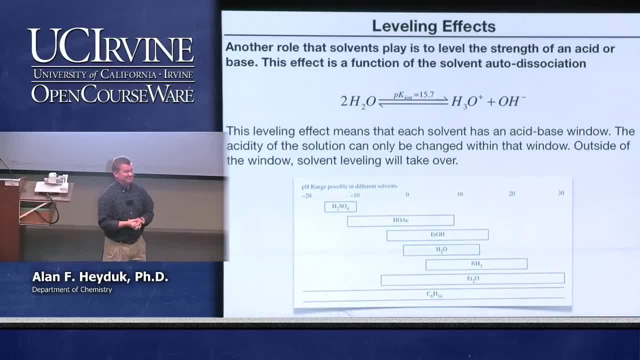 of a proton from hexane. Nah, If you put that on your final in 51B, not good stuff, Right? And so there is no ionization of hexane, right? If you dissolve a strong acid in hexane, if you can get it to go in. 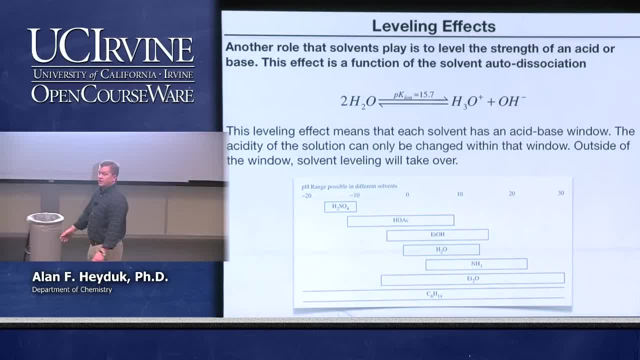 you're going to get protons and whatever the conjugate base is Okay. There's no leveling effect in hexane because it can't dissociate under. you know, on this planet at least, Maybe if you go to bizarro world, things are different. 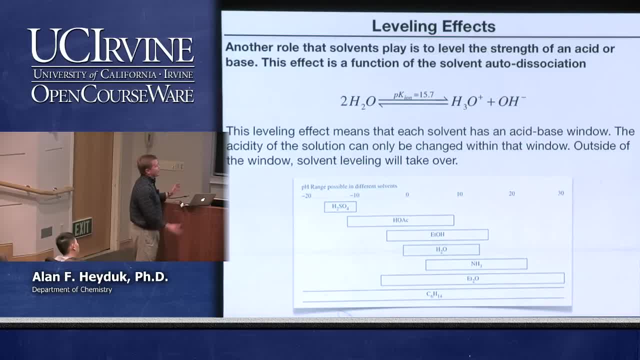 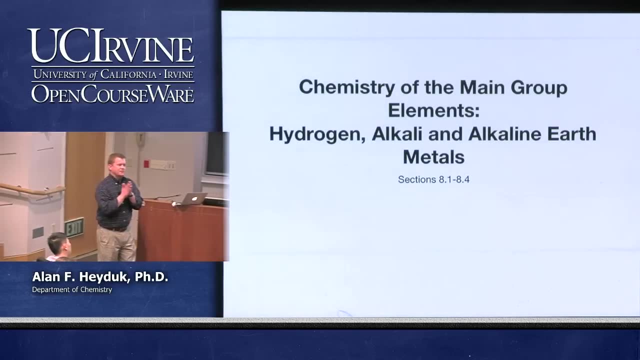 But on this planet, hexane doesn't dissociate, And so there's really no, there's no leveling effect, and there's no limit on the basicity or acidity of a solvent or of a solution that you can make. Okay, So that's the end of the acid-base chapter. 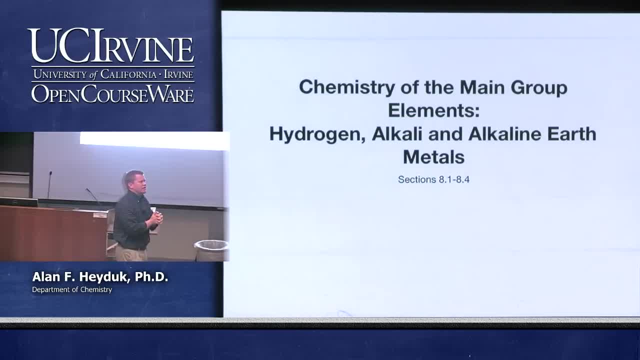 which I want to stress to you. A lot of that stuff seems incredibly trivial, right, Like: why are we juniors and seniors at UCI and talking about acids and bases? okay, But so much of chemistry is acid-base driven okay. 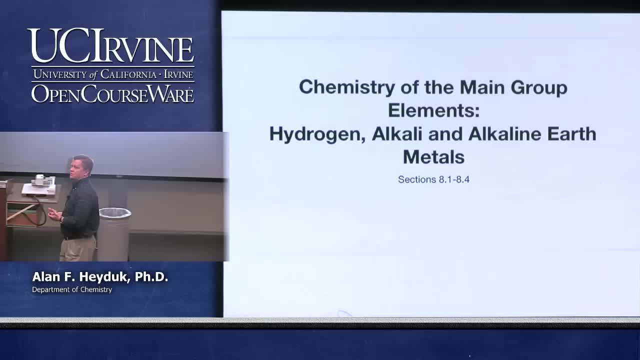 Every time in Chem 51 you heard about a new, a nucleophile. you could just substitute the word base, Electrophile, Lewis acid. Okay, It's all acid-base chemistry, or a good portion of organic chemistry is acid-base chemistry. 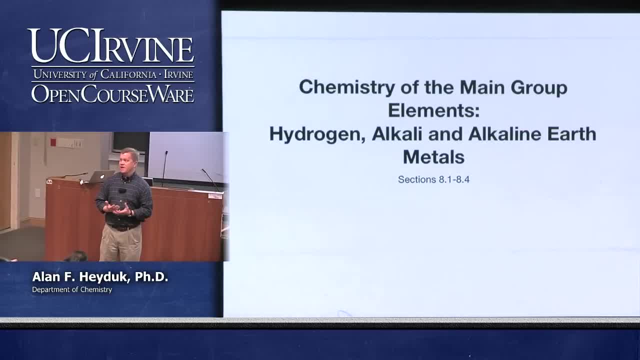 An incredible portion of inorganic chemistry is acid-base chemistry. Okay, These may seem like simple fundamentals and oh, it's just freshman chemistry, But trust me, you master that you're going to be a long way out. Okay, You're going to be a long way to doing very well. 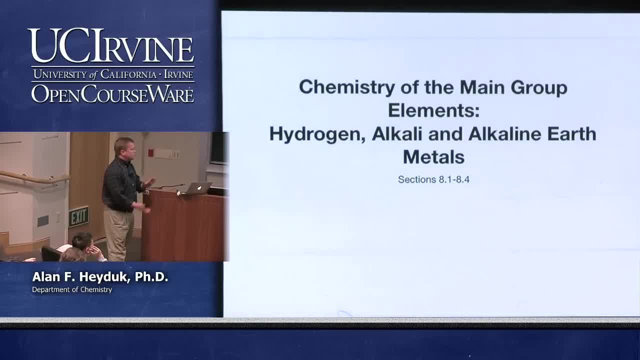 in all the rest of your chemistry courses. So this next chapter that we're going to cover, chapter eight, is. I promise it's the only chapter that we're going to do like this. It's what we would call descriptive chemistry, And what we're going to do is a very quick periodic march. 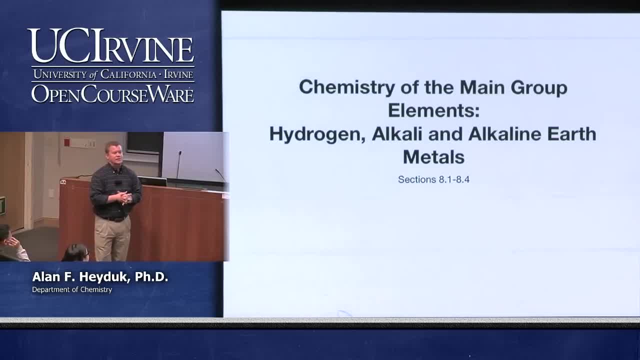 We're going to start with hydrogen and we're going to kind of walk across the periodic table, so I can just give you a flavor of the chemistry that is possible with some of these elements that you haven't talked much about in your chemistry careers up to this point. 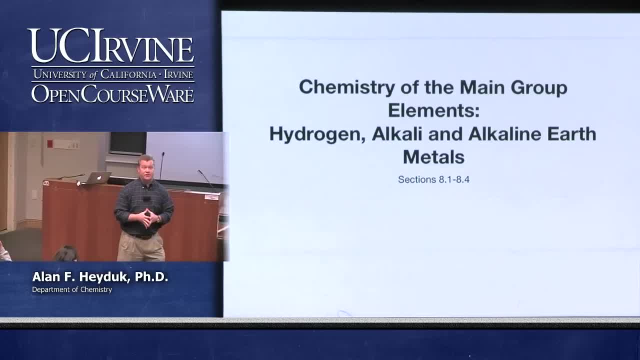 Okay, Again, I want to calibrate you. We're going to spend roughly three 50-minute lectures on this, minus what we've already spent today on this. You spent three quarters talking about the descriptive chemistry of carbon in Chem 51.. Okay, So I'm probably not going to touch on everything. 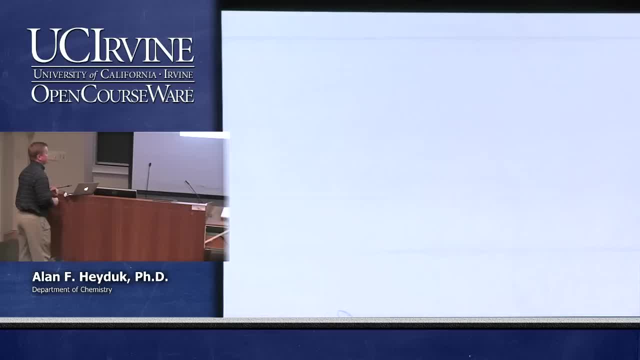 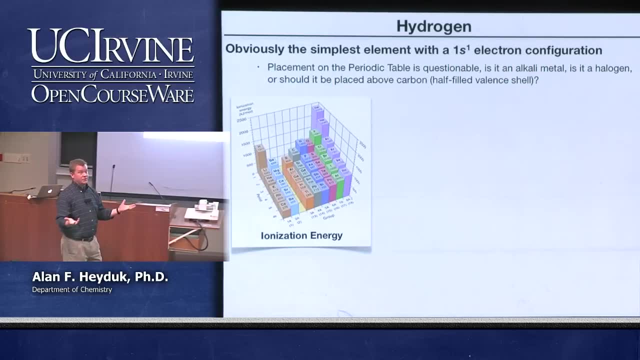 Forgive me. Okay, Hydrogen. How interesting can hydrogen be, right? It's got like one proton and one electron. Okay, Okay. So let's first talk about where it's located in the periodic table. It's that top left corner. 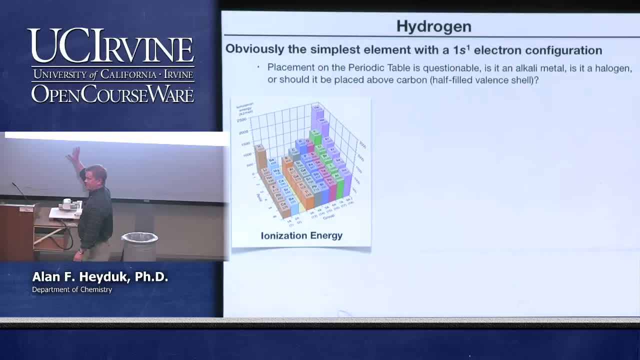 I mean this is a truncated version of the periodic table. They've cut out all the interesting elements, which are the transitions. We'll get to those later. But we all know that hydrogen is always put in that top left corner, right above lithium. It's the first element, But why? Well, because it has one proton and one electron and a 1s1 electron configuration. But if we look at the ionization energy- remember the ionization energy is the energy required to pull that electron off of a hydrogen atom in the gas phase. 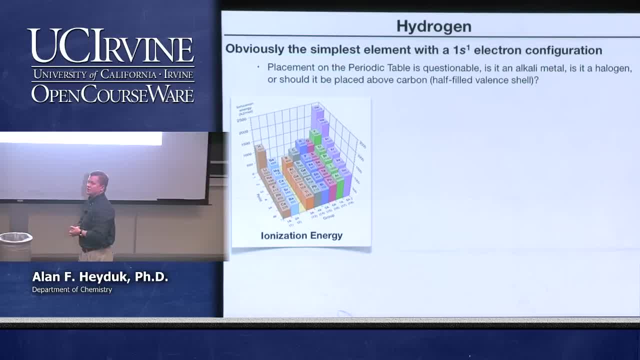 Well, it may be too small for you to read, but it's 1,311 kilojoules. It's over twice as large as the next element down in the periodic in its column, And in fact it's comparable to oxygen. 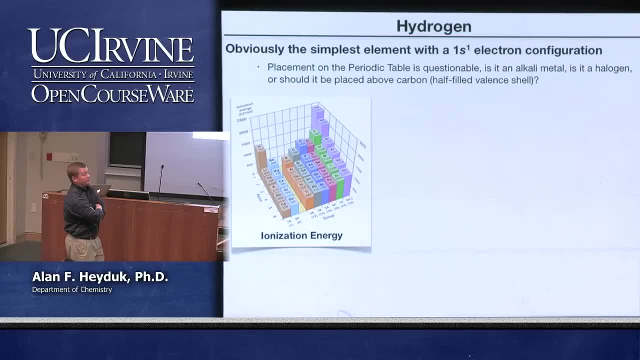 Well, that's weird. So it's not quite as high as fluorine. Fluorine is about 1,681 kilojoules, But oxygen is 13.1.. 1,314.. So it's close. So why again did we put hydrogen all? 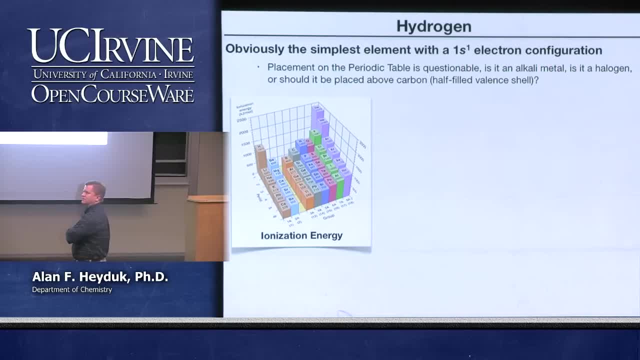 with these electropositive elements. Maybe really where it belongs is above fluorine And if you think about it, that's okay, because it only needs one more electron to close its shell. Okay, We can look at electrons. We can look at electrons. 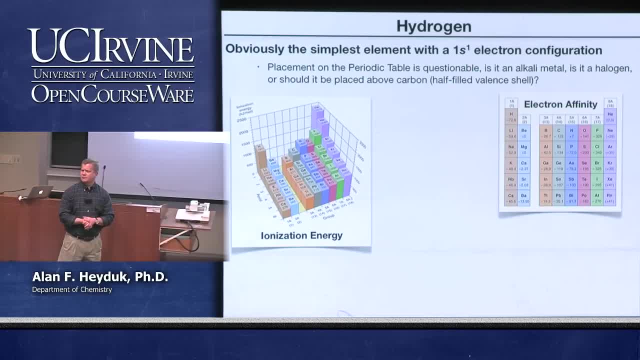 We can look at electron affinities And then we realize it really doesn't belong above fluorine. Fluorine has an electron affinity of minus 328 kilojoules, So it really really, you know, it's really happy. 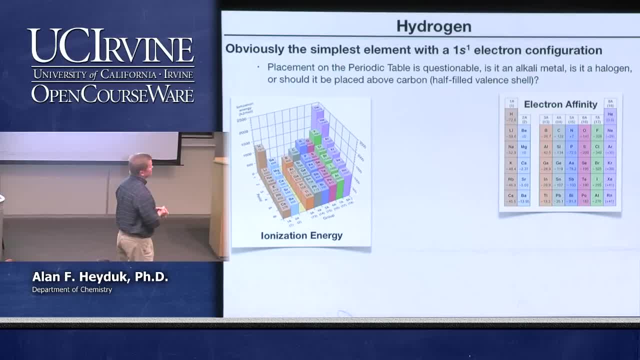 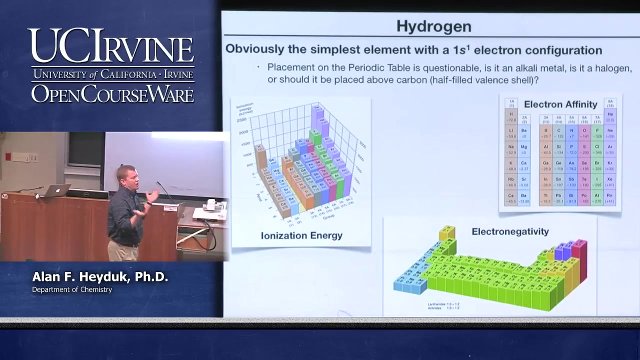 to take on an extra electron, Hydrogen minus 73.. Looks like it actually fits really well right there with those other alkaline metals. But now we go back to the electronegativity, And this is a number we should all have. 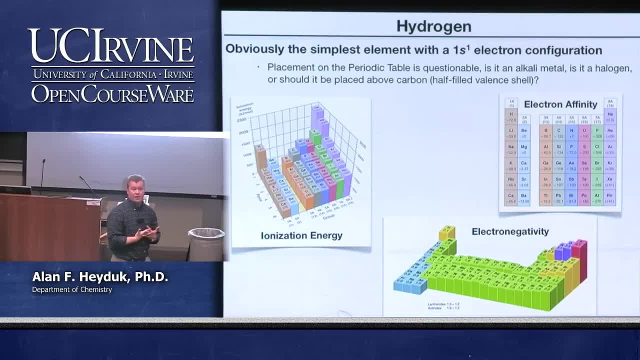 be pretty familiar with right, Because we know that carbon-hydrogen bonds are pretty much covalent. They're not polarized very much. So that means hydrogen must have a similar electronegativity to carbon. Sure enough, it does. 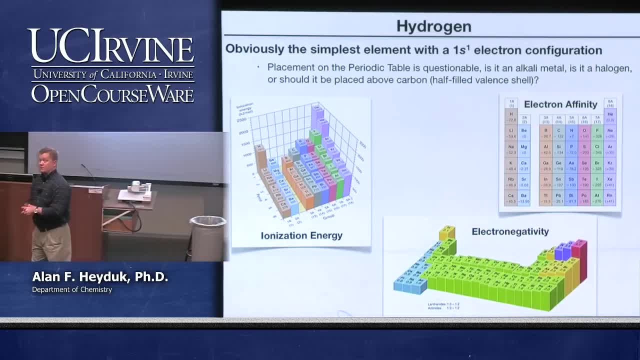 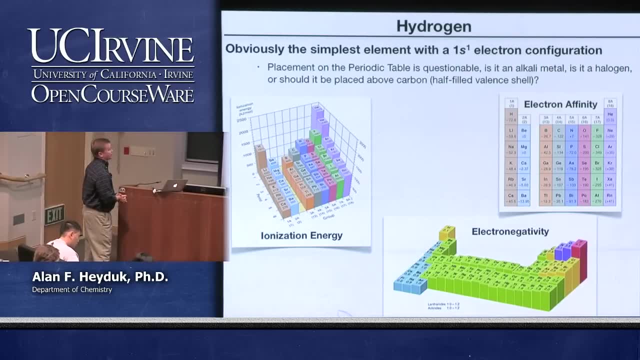 2.1 to 2.5.. So it looks again more like one of these p-block elements than it does one of the alkali or alkaline earths where we're seeing. I guess beryllium has an electronegativity of 1.8, but lithium is at 1.0. 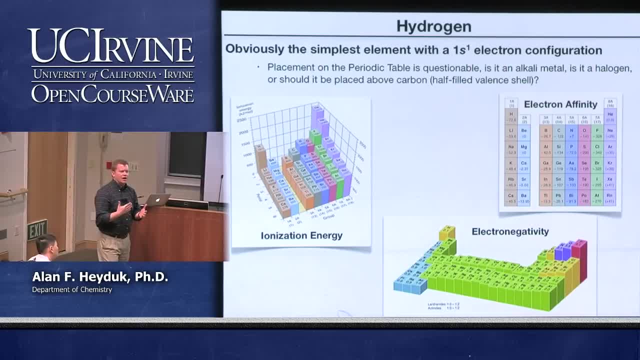 Electronegativity, remember, is the measure of how willing the element is to share its electron in a covalent bond, So it's kind of like ionization energy It's. I'm sure there's some formula somewhere that relates them, but it's not the same. 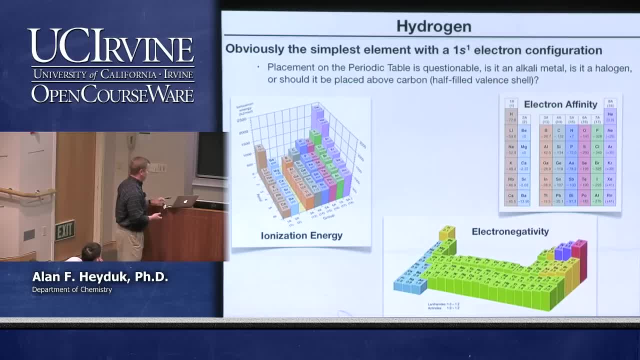 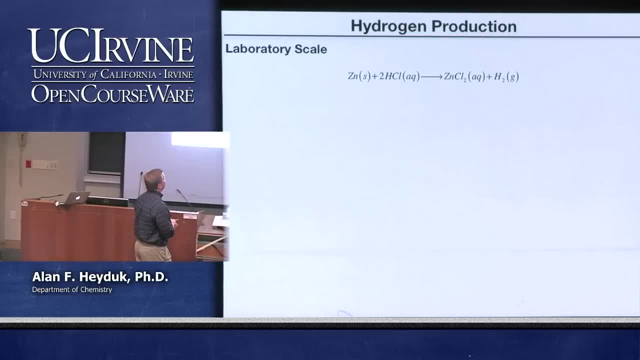 So hydrogen is kind of a strange beast, which is good because it's a pretty important element. So how do we make hydrogen in the lab? It's fun. You take aqueous hydrogen chloride, drop in some zinc, metal bubbles, start coming off. 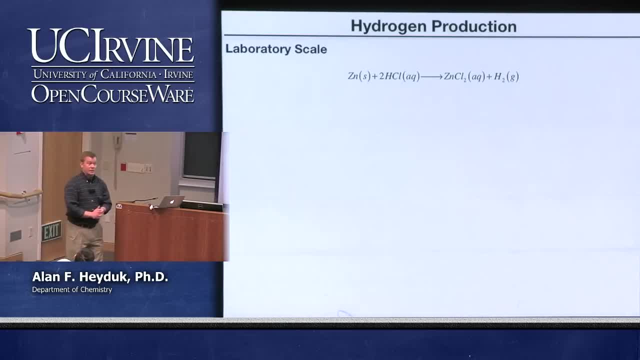 There you go. That's not a very practical Way to make it on a large scale, I guess, unless you have, you know, a zinc mine in your backyard. Turns out that the way we make it on an industrial scale is called steam reforming. 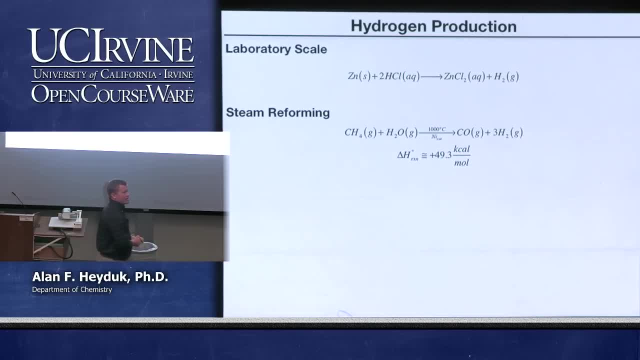 And so this is a cool reaction to me. You take methane and you take water- Oh god, I hate these cameras- And you heat the crap out of it. That can be edited right. You heat it up. You can heat it up. 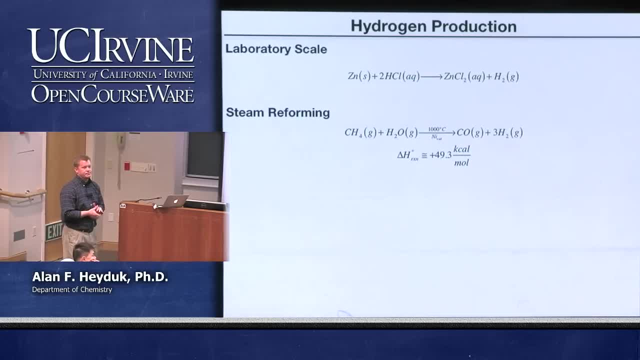 You can get out carbon monoxide and hydrogen. Or if you live in Kentucky, you say you want to do this with coal, And you take coal and you heat it up with water and CO comes off and H2 comes off and you separate them. 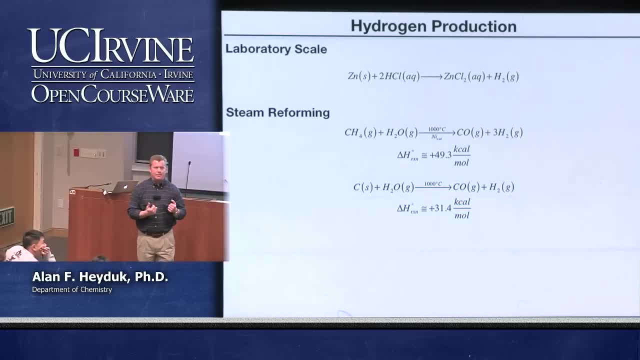 Now you've got your hydrogen. Now what's interesting about both of these reactions? Well, they make carbon monoxide, That's. that's, yeah, poisonous, you know? Eh, come on. Yeah, look, these are both endothermic reactions, Not just a little bit endothermic. 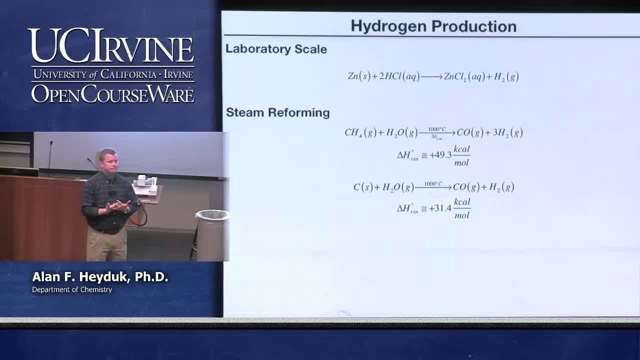 A lot endothermic. So what drives the reaction? Bubbling of gas? Did somebody just say equilibrium Heat? There's a? there's a thermodynamic state function. It's, it's our favorite one. It's the one we used with our parents. 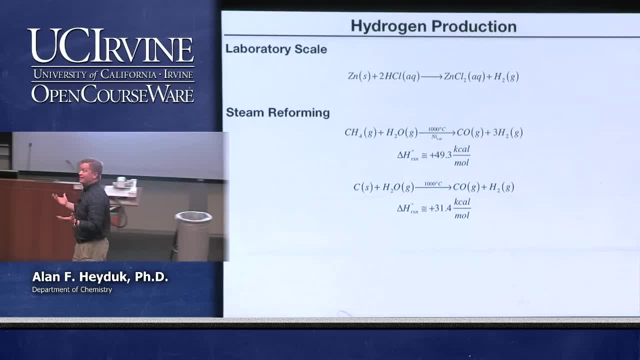 when we didn't want to clean our room. right, Entropy, right. So entropy drives this reaction. right. We do this again. recurring theme: Simple freshman chemistry On the left hand side. let's, let's make it the most stark. The second reaction: for coal, we have one mole of solid. 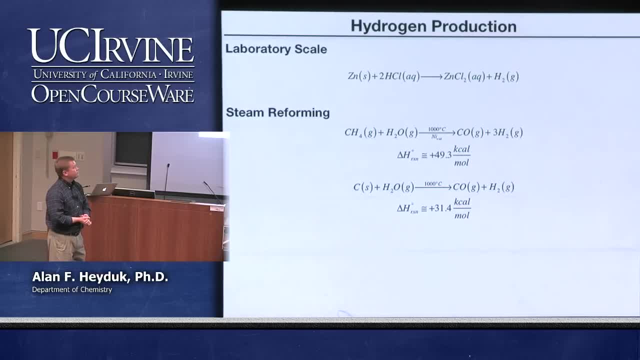 And one mole of gas, going to two moles of gas, That is, and you get a massive increase in entropy because you're making more gas in the product than you are, than you have in the reactant, Which is why we run the reaction at a thousand degrees. 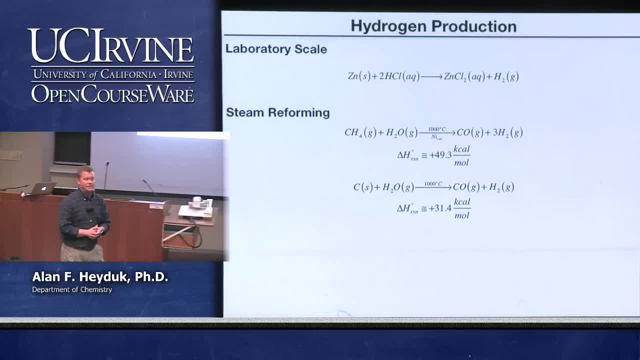 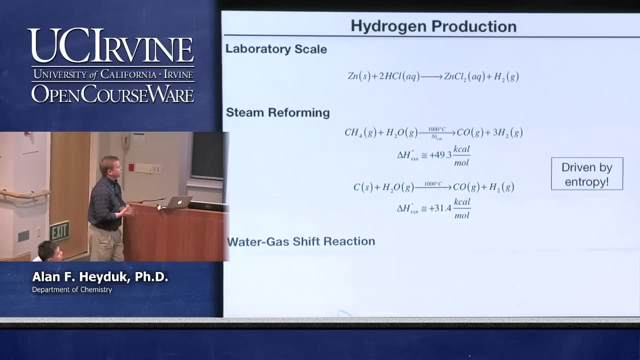 Remember, delta G is delta H minus T, delta S. So if T is a really big number, in this case 1,273 Kelvin, You can overcome that positive enthalpy. And for those of you that were worried about carbon monoxide, That was figured out too. 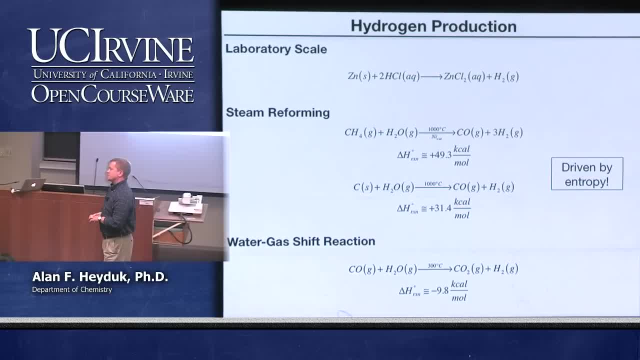 It's called the water gas shift reaction. You take carbon monoxide, heat it up with some more water, Get out CO2 and another equivalent of hydrogen. That one's downhill slightly about 10 K cals per mole, Which is good, because the entropy is more or less a wash. 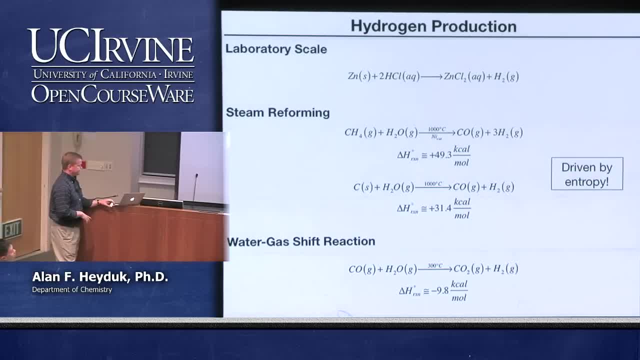 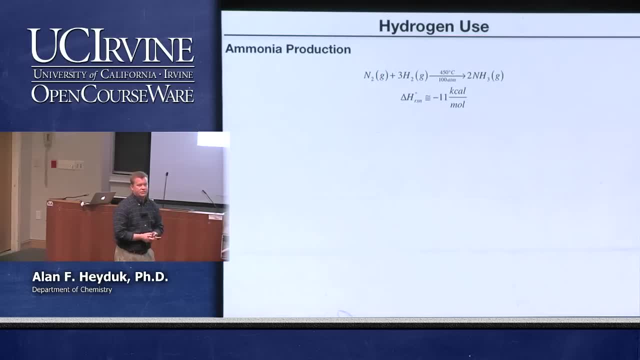 Okay, So that one is enthalpy driven, All right. Where do we use hydrogen? The number one source- industrial- of hydrogen use is in making the food that you eat, So you take. we use hydrogen gas to reduce ammonia or to reduce nitrogen to ammonia. 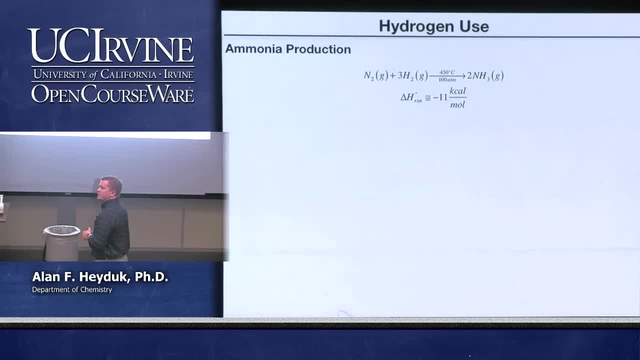 I think you've heard- probably heard some of these numbers before. Roughly 40% of the nitrogen atoms in your body went through the Haber-Bosch process And we're fixed in this way. Okay, This is why roughly half the world can eat. 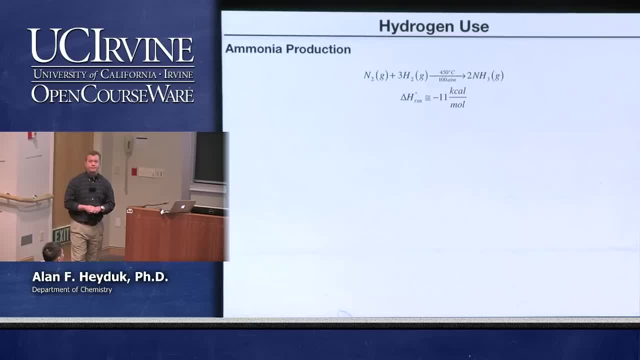 Is because we're very good at doing this reaction. Okay, I think it's the only chemical reaction that was awarded two Nobel prizes, Okay, One for the actual chemistry And one for the engineering that allows you to do it at 450 degrees Celsius and a hundred atmospheres of pressure. 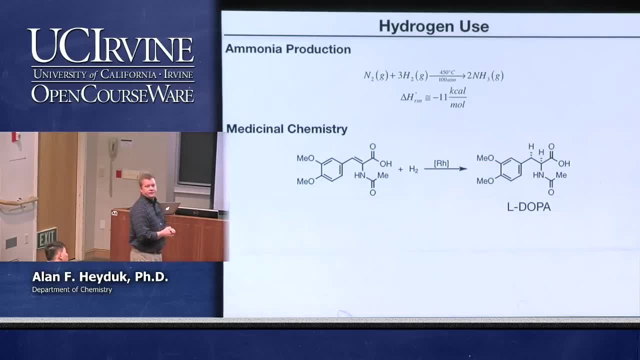 Where else is it used? Well, we of course learned lots about hydrogenation reactions in 51.. Here's a really, really famous one. So L-DOPA was discovered like 50 years ago And it's anti-Parkinsonian effects were well established. 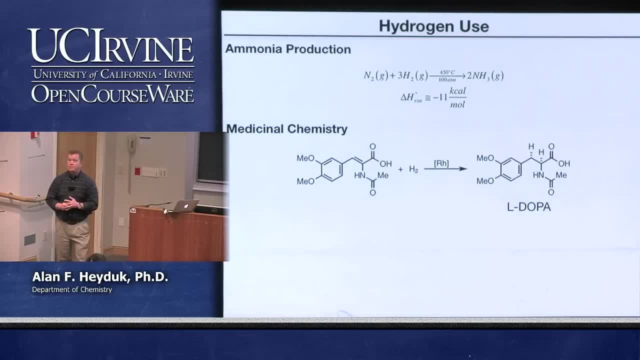 The problem was we couldn't make it Okay Until an organometallic chemist designed a chiral rhodium catalyst to perform the hydrogenation of that internal olefin in a stereoselective way. That reaction goes with about 99% stereoselectivity. 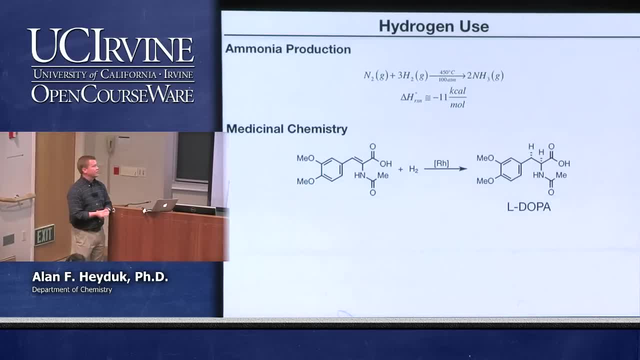 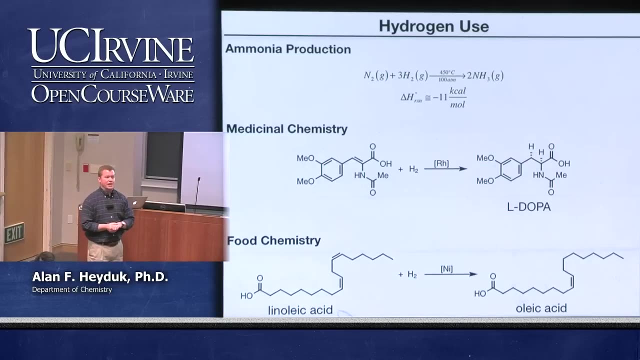 And it allows any patients with Parkinson's to now get L-DOPA at a reasonable cost- Nobel Prize in 2001.. We use it in food chemistry Also. who's heard of hydrogenated oils, right, Well, so why do we do it? 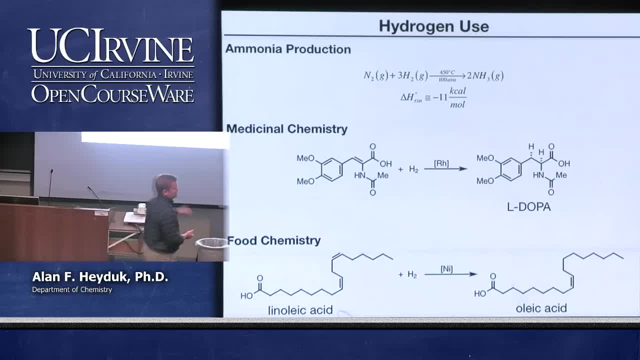 Well, because some brilliant chemist said: hey look, our product has linoleic acid in it. It's an omega-9.. It can be inflammatory. It's not really good for you, But if we hydrogenate it with a nickel catalyst, 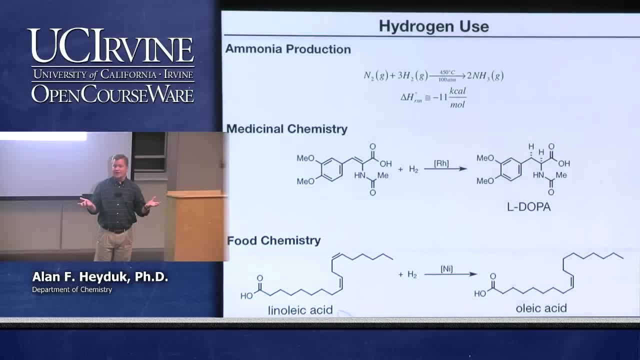 we make oleic acid. Where do we normally get oleic acid? Olive oil, Olive oil, right, That's the omega. oh, no wait, this is an omega-6, sorry, Linoleic is an omega-6 and it's inflammatory. 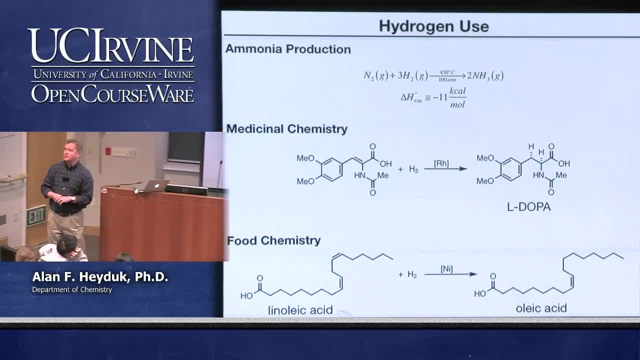 Oleic is an omega-9 and it's considered one of the essential fatty acids. that's really good for you. Of course, when we do the hydrogenation chemistry it gets turns out that we're not as good at doing it as mother nature is. 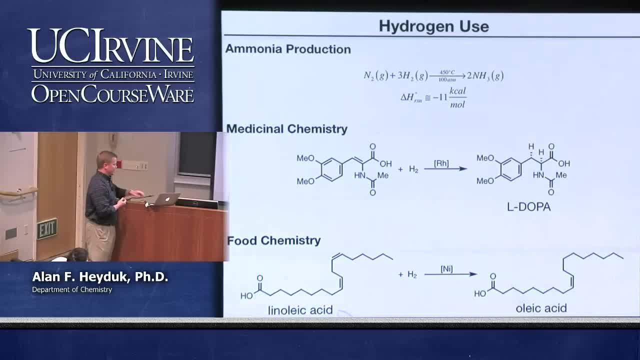 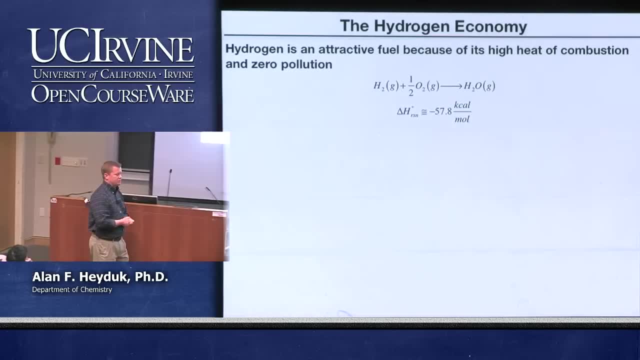 So You're better off getting your oleic acid from real good olive oil. Plus, it tastes a whole lot better. Okay, so the hydrogen economy, alternative energy, is a question that's near and dear to my heart. Several of you are probably way too young to remember one. 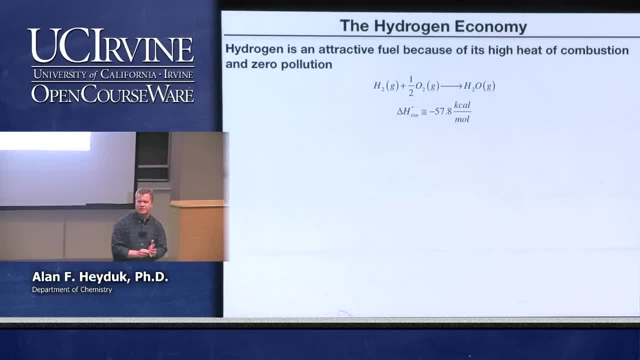 of our former oil-loving presidents getting up in front of Congress and talking about the hydrogen economy and how fantastic it was going to be and why you know it was so good, because all that would come out of the tailpipe of your car was water. 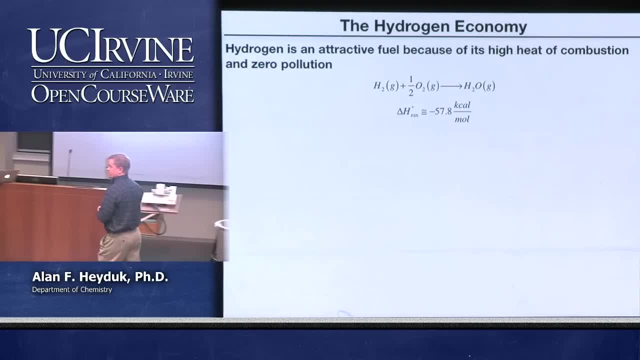 It's fantastic, right? You burn hydrogen in the air and you get water out, No pollution. It's fantastic. Well, sometimes you have to dig just a little bit deeper and you have to ask yourself where to again. where does that hydrogen come from? 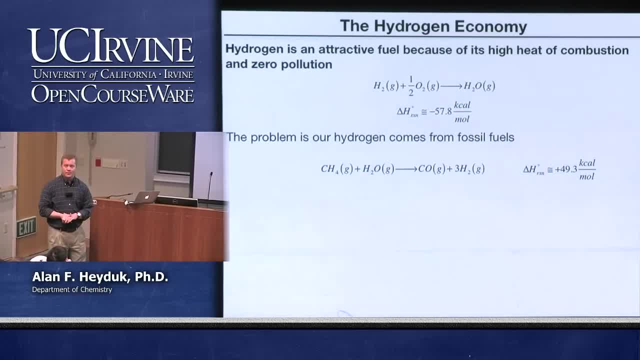 And we already told you where it comes from: Steam reforming. So if you take methane and water to make your hydrogen, you get off CO. It's uphill. Then we take the CO and we do the water-gas shift reaction to make CO2, we get another equivalent of H2 out. 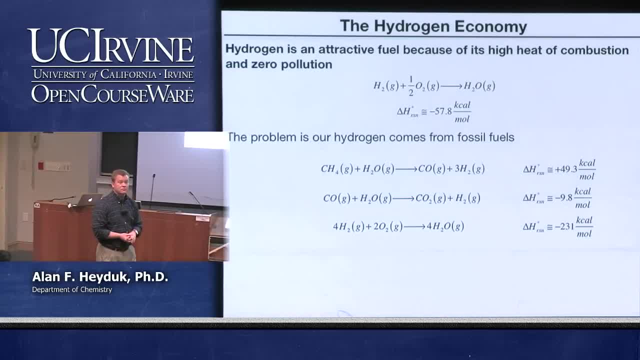 Well, and then we take that hydrogen and we put it in your fuel cell car and we use a fuel cell, and with high efficiency, let's say we burn it to power your car, We get out water. That's all that comes out of the tailpipe. 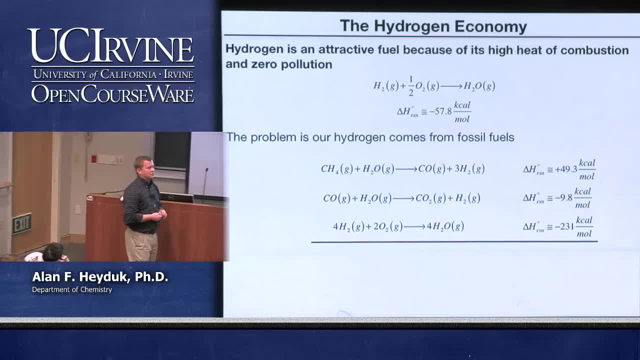 But again, we're chemists and we know that we're going to get water out of the tailpipe. It doesn't really matter how you get from start to finish, what steps you go through to get there. All that matters is what you started with. 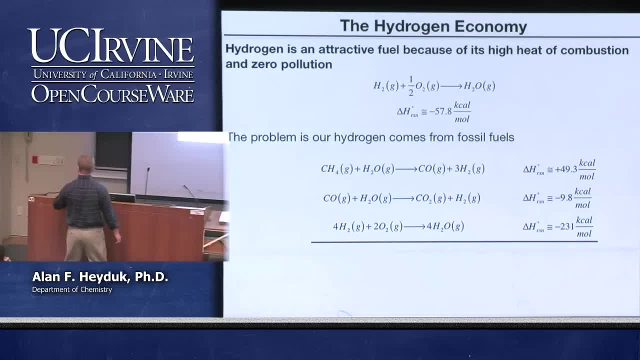 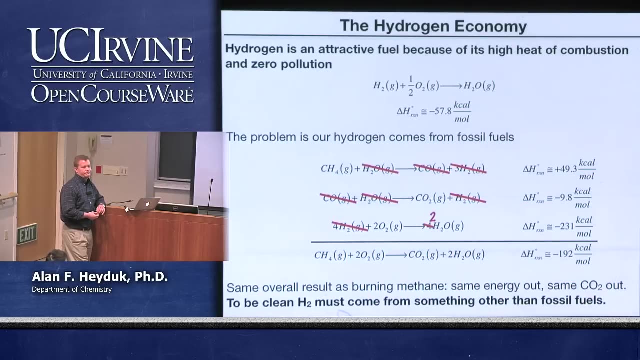 and what you ended with. And in this case it doesn't matter whether you directly burn the fossil fuel or whether you go through this chemistry exercise of turning it into hydrogen and then burning it. your net reaction is the same: Methane plus two oxygens goes to CO2 and water. 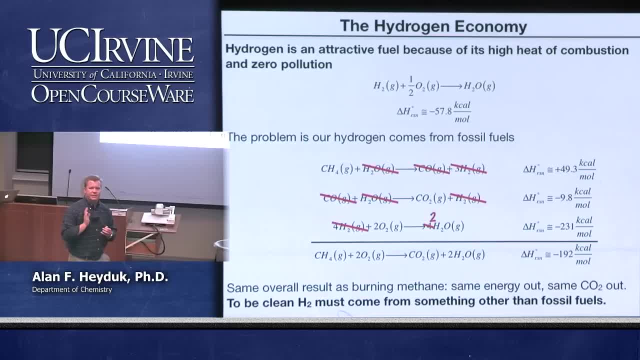 Okay. So I say this because you guys have the tools to think about these things and it's critical that you do. Okay, A hydrogen-powered car that gets its hydrogen from oil or natural gas or coal is really no cleaner than a gas-powered car. 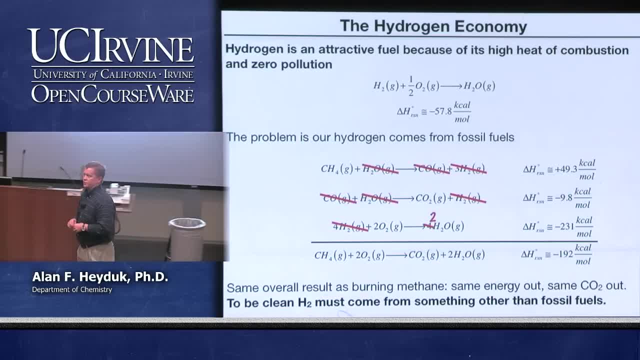 It's just you're changing where the CO2 is produced. You produce it at the factory that makes the hydrogen rather than out of your tailpipe. Now there are some chemical engineering questions about whether it's easier to deal with the CO2 at the factory. 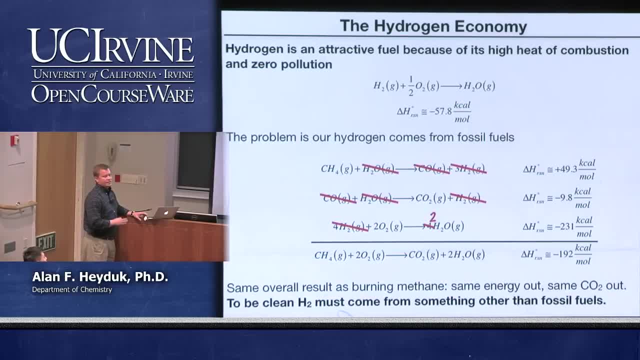 but the chemistry is very clear: You get the same amount of energy, You get the same amount of pollution. What we really want to do is generate hydrogen from something other than fossil fuels, And if you're interested in those concepts, I'd be happy. 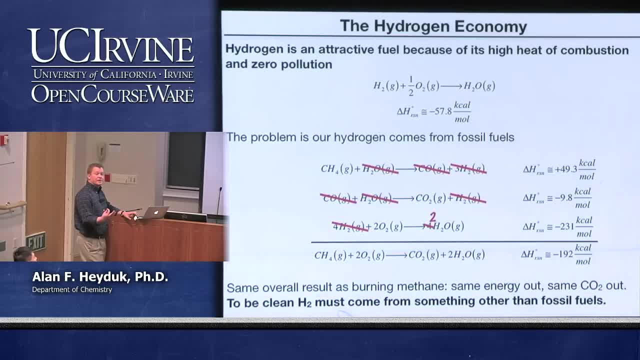 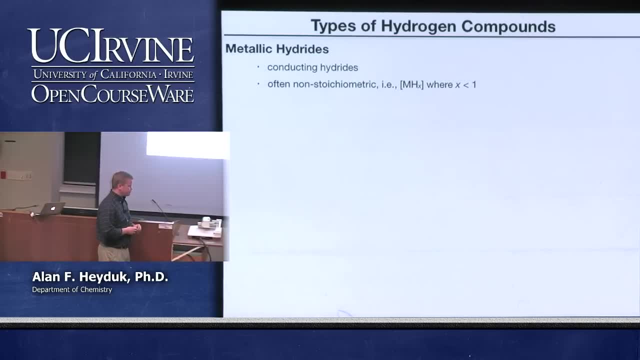 to talk to you about it. My research is geared toward it, So is Professor Law's, And so both of us have a vested interest in understanding that kind of chemistry. Okay, But again, descriptive chemistry. What other kind of hydrogen compounds are there? 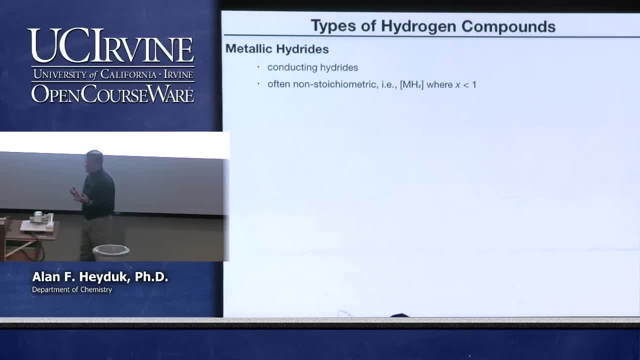 Well, one are the metallic hydrides And, frankly, these are not. they're very interesting compounds, but they're hard to discuss because they're non-stoichiometric. Okay, And so you can get hydrogen to react. You can react with various metals and make these species. 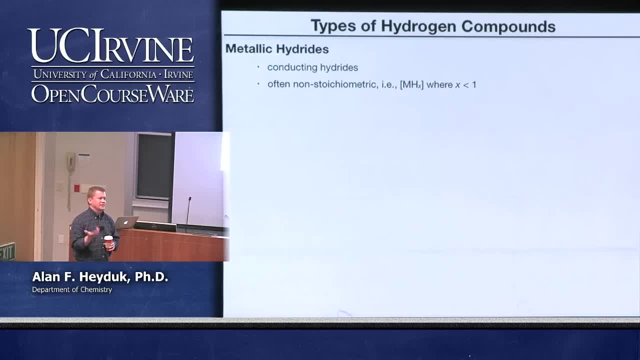 that have MHX-type formulations where X is some number less than 1.. Okay, And we all know as chemists that it's kind of hard to study and talk about compounds when we can't put a real definitive formula on it. Okay, Or know the structure. 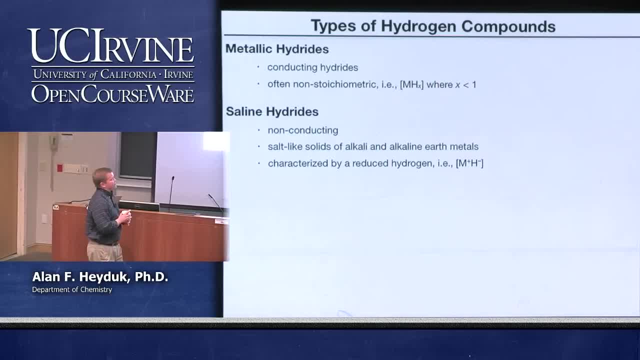 So we aren't going to talk much about those. There's the saline hydrides, okay, where you basically have a hydrogen compound of an electropositive Okay. So these are salt-like solids and they're primarily the alkaline. 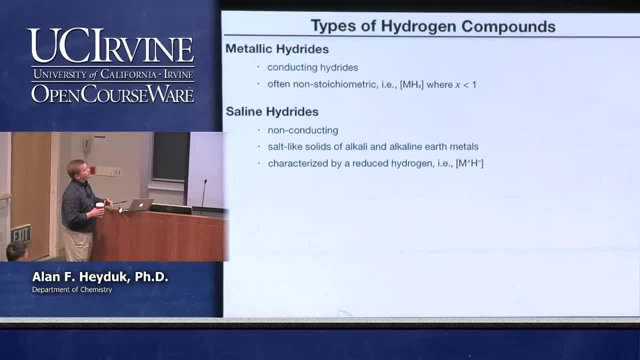 made with the alkaline and alkaline earths And we can describe these as hydritic compounds. So these are compounds where the hydrogen actually looks like H minus a closed shell species. It's kind of acting almost like a halogen by binding. 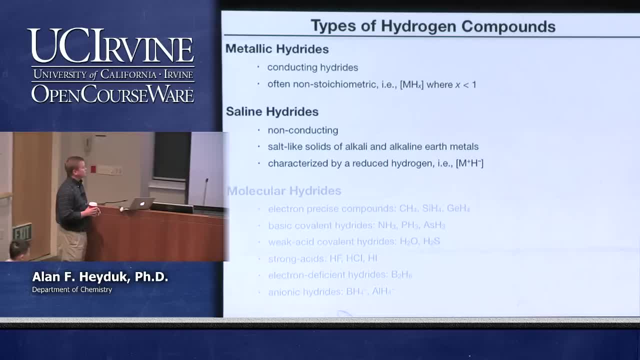 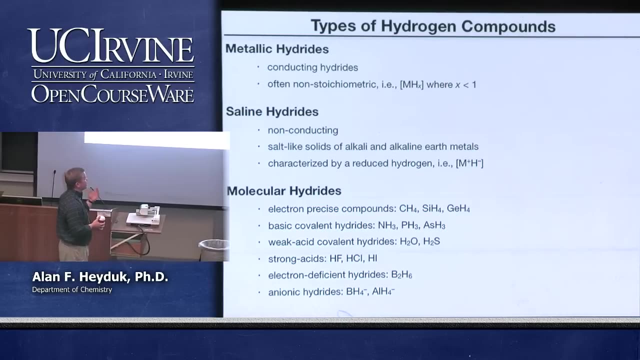 with an electropositive metal. And then there's the molecular hydrides, So these are the hydrogen compounds of the P block elements. We're, of course, all familiar with methane. It's great. Okay, These are what we call. it's an example. 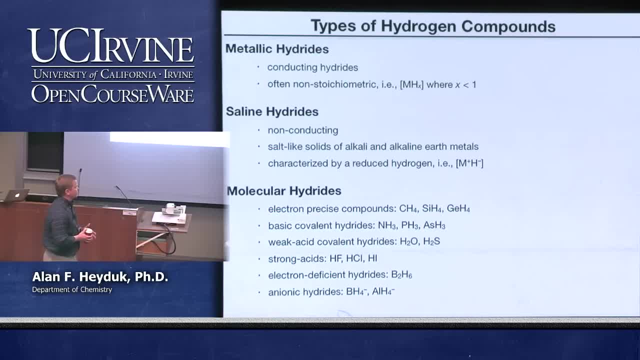 of an electron precise compound, So it's characterized by highly covalent, bonding, symmetric structures. There's exactly one hydrogen atom for every valence electron in the central P block element. all right, four hydrogens. Carbon has four valence electrons. 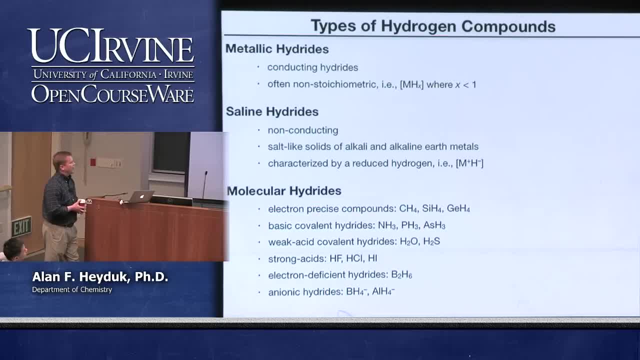 Everything works out nice. We have the basic covalent hydrides, which are one step over, So, ammonia being the prototypical example. Phosphine and arsine are also examples We have if we take two steps from carbon. 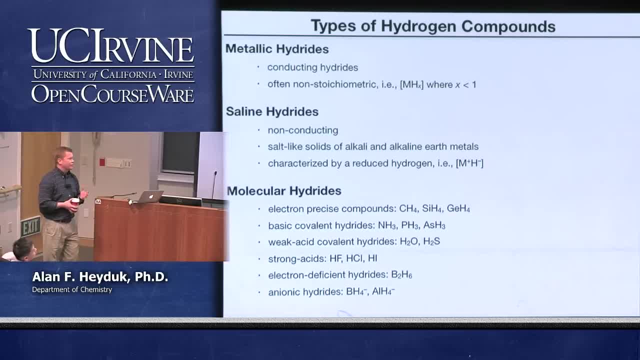 we have the weak acid, covalent hydride, So now we have water hydrogen sulfide. These are species where there's two lone pairs and two element hydrogen bonds And then the strong acids, So the hydrogen compounds of the halogens. 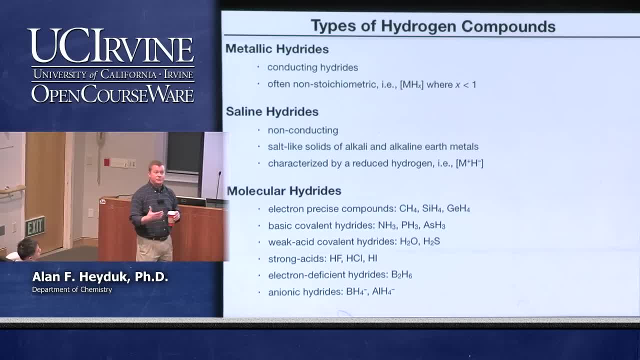 So in the saline hydrides I said that hydrogen was kind of almost acting like a halogen by accepting an electron from an electropositive metal. Now we see we have the strong acids where hydrogen acts as the electron. it acts like an alkali, alkaline metal. 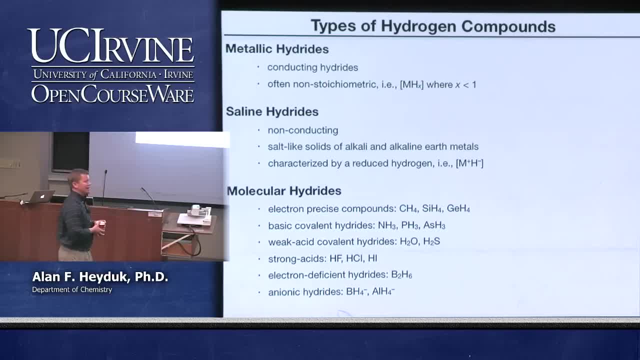 and gives up its electrons to the halogen. okay. So again, hydrogen really is is special in that it can can act in either way. The electron deficient hydrides are really neat. So instead of taking a step to the right from carbon, 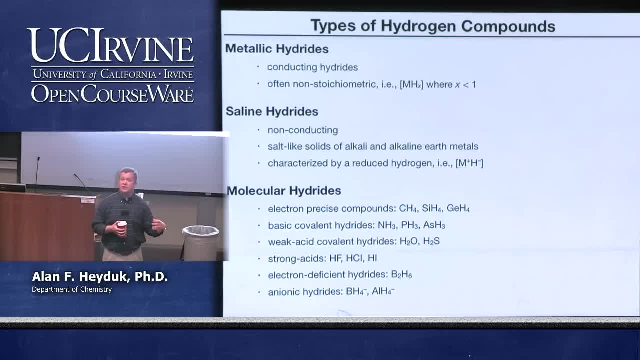 from the precise hydrides. we take a step to the left. We're basically removing one electron from the central p block element. And now, when we make the maximum number of covalent bonds, boron can take three hydrogens because it has three valence electrons. Well, we all know that the problem with BH3, is that it's not going to be as good as hydrogen. So we're going to have to take a step to the right from carbon. We're going to have to take a step to the left from hydrogen. 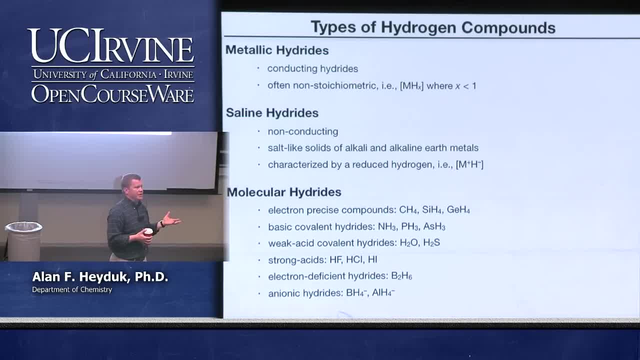 So we're going to have to take a step to the right from carbon. Again, it's a freshman chemistry problem is there's not a complete octet right. BH3 only has six electrons around the central atom, and so it does things like try to pick up another hydride. 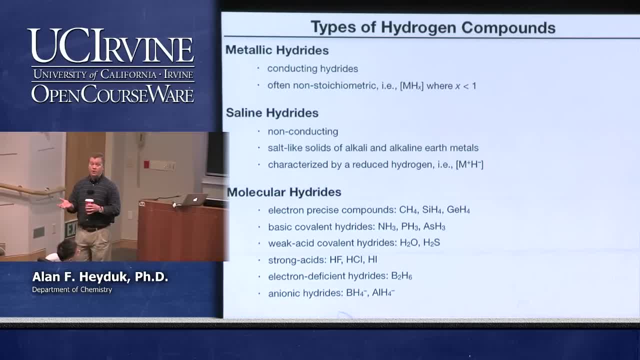 And so that's where you get BH4.. So sodium borohydride is a common reducing agent in organic laboratories. okay, Because it's a source of hydride ion. If you want a little bit more oomph, you go. you make the aluminum hydride. Lithium-aluminum hydride is a more powerful reducing agent, So again, can you tell? I love freshman chemistry. So we measure the stability of these hydrides by looking at heats of formation, right? 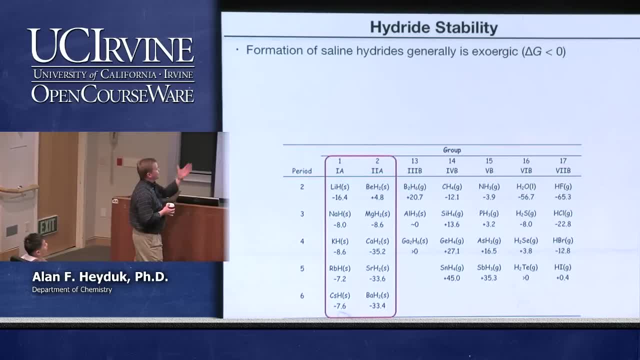 And so we can look at the saline hydrides- Remember, these are the ones for the alkaline and alkaline earth metals- And you'll notice that largely the formation of these hydride complexes is exoergic. okay, So exothermic is a negative. delta H- Exoergic is a negative. 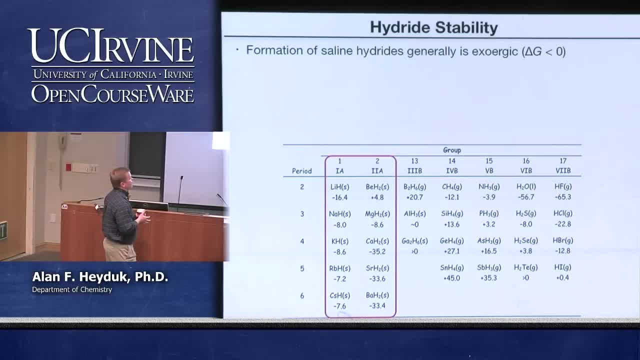 delta G. So there's a. it's a negative free energy of formation for these hydrides, with the exception of beryllium hydride. So one thing you might say is that these are pretty stable, okay. The other thing is to keep in mind. 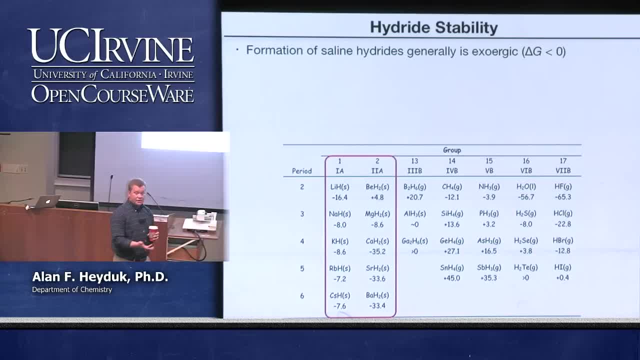 when we say they're exoergic. free energy has two components. It's got the enthalpy component and it's got the entropic component. When we talk about a heat of formation of a compound, we're talking about the heat of formation from pure elements. 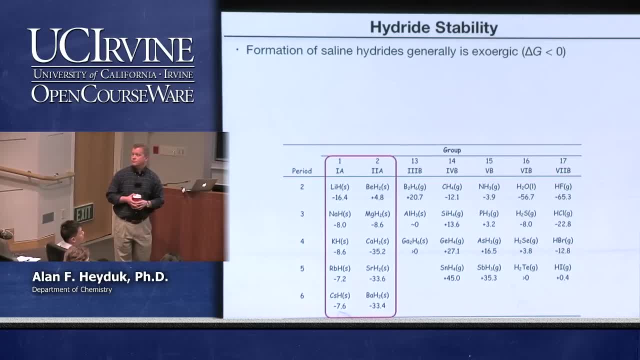 Well, if we make lithium, well we're making it from lithium, which is a solid- it's a metal- and hydrogen, which is a gas, And now lithium hydride in its standard state is a solid. So we're getting kind of a big entropic thing. 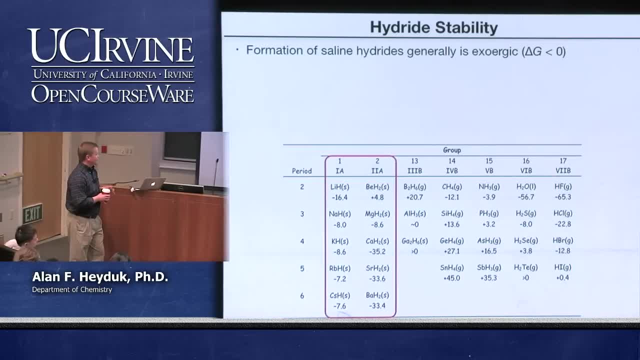 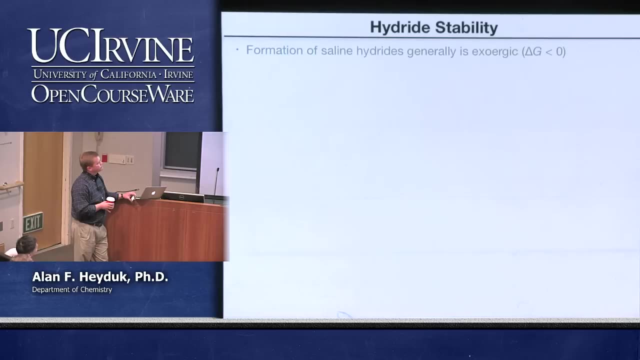 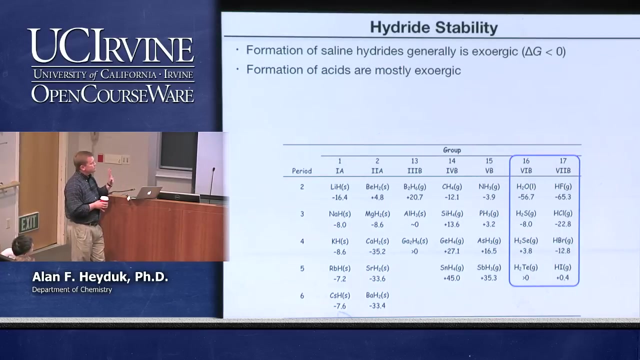 There's a big entropic component that is incorporated into that negative delta G number. Okay, Whoops, I didn't mean to do that. Sometimes, There we go. Okay, The acids. this is probably going to come as no surprise. 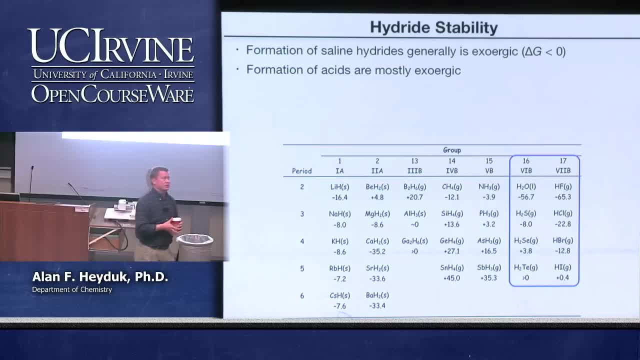 These all pretty much have negative heats of formation or sorry, they're exoergic free energies of formation. We all pretty much know that water is a pretty stable compound, Right? So it's not surprising that it has a very negative free energy of formation. 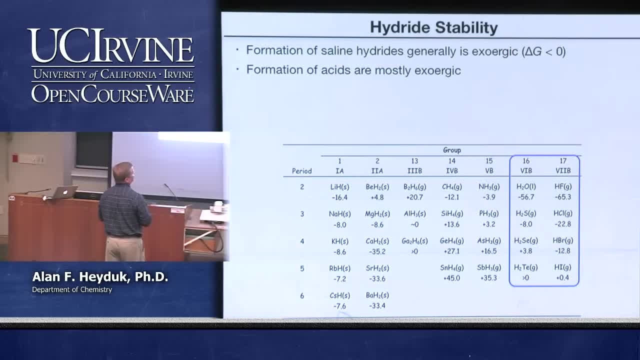 HCl: same thing. There are a few exceptions. Okay, Hydrogen dihydrogen selenide is slightly positive. HI is right around zero. Okay, And so HI, if you have it, it can decompose to. 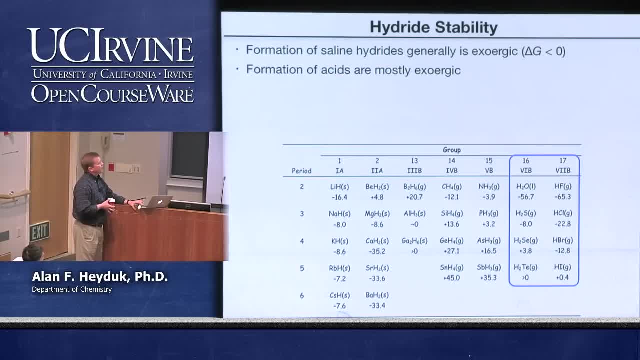 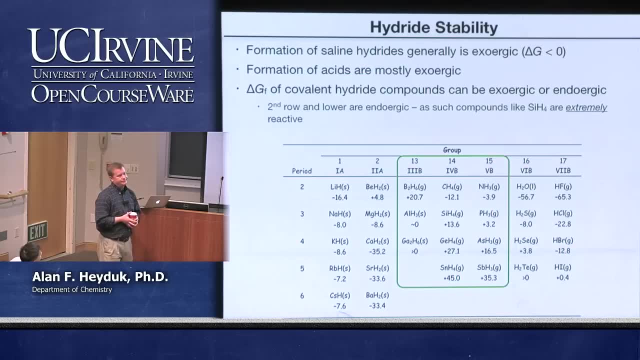 it's about thermo-neutral for it to go to hydrogen and iodide. So though, there is a pretty decent kinetic barrier, And then there's the rest: The electron precise, the electron deficient. the basic covalent hydrides can either be exoergic or endoergic. 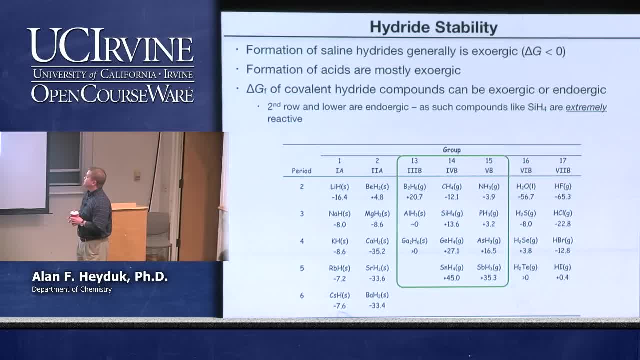 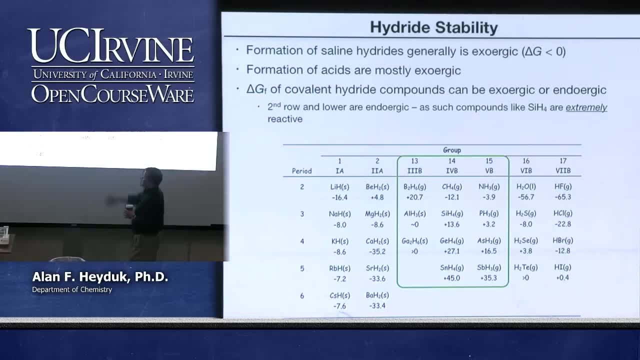 You'll notice where the break point really seems to be. The electron deficient are a little bit odd because again of this idea that you don't have the completed octet. But you'll notice methane and ammonia are, both have negative delta Gs of formation, but all 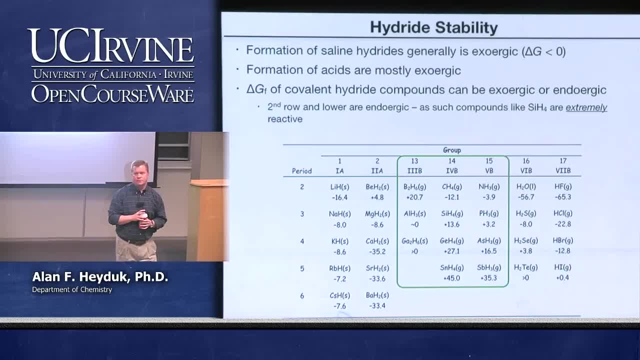 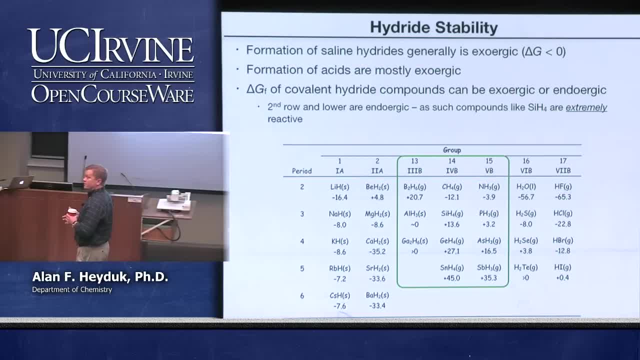 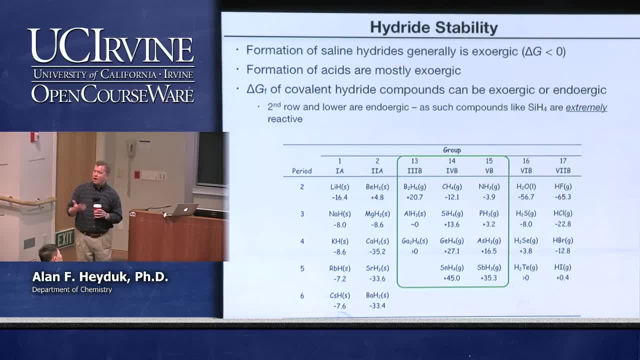 Okay, Okay, And again, this is something you can probably rationalize using your freshmen chemistry knowledge. right, We're taking a pretty small 1s orbital and trying to make a bond with now a 3p orbital. Okay, Basically it becomes a hard, soft acid-base problem. 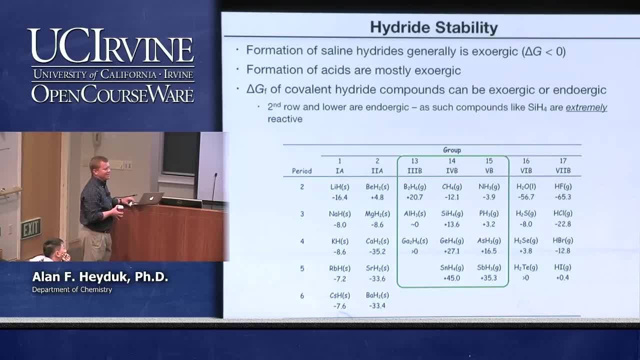 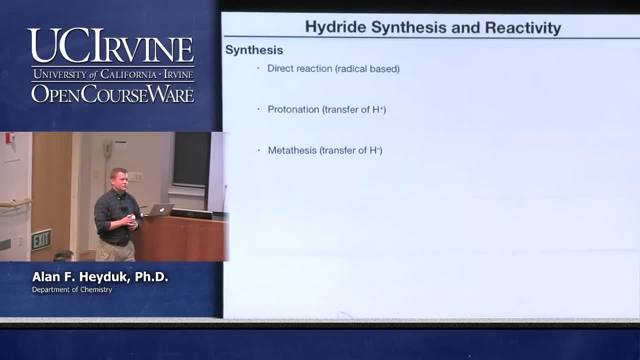 Did I just say that? Geez, yeah, I guess acids and bases are important. Okay, so this is one of my favorite slides because it's really redundant. How do we make these hydride compounds? Well, there's three basic reactions. 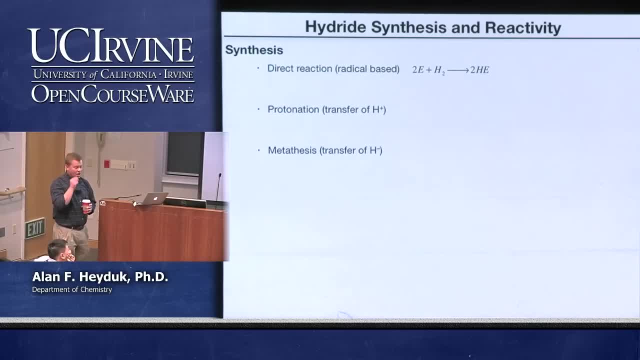 The first is a radical process where you take basically two of the element and react it with hydrogen gas and make the corresponding element hydride. So this is written in a very generic way. Has anybody ever seen the reaction, the demonstration where you react hydrogen gas? 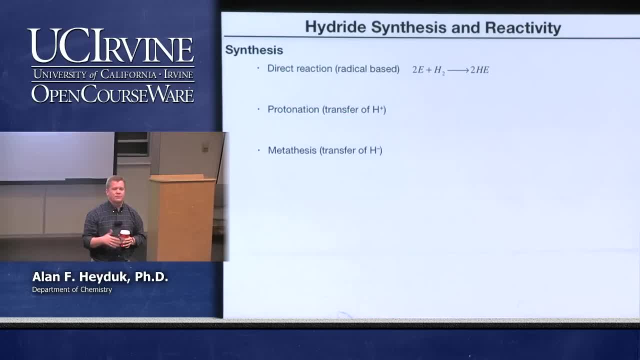 with chlorine gas. See, okay, between you and me and the millions of people that will be watching us on video on YouTube, this is what I don't like. We should have demonstrations, because that's what makes science cool, So I'll tell you how it goes. 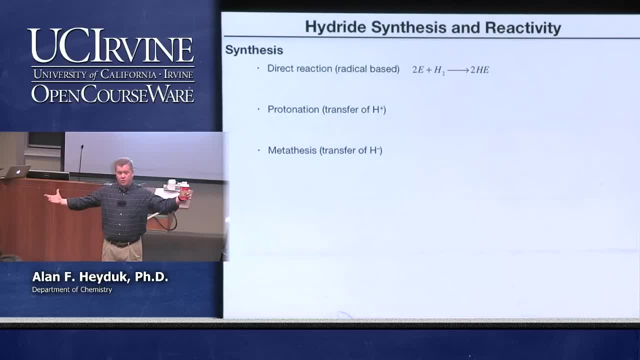 So you get a big quartz tube, quartz glass tube, and you fill it with a mixture of hydrogen gas and chlorine gas. Chlorine gas is this faint? it's very, very, very faintly green. You put quarks on either end and it sits here. 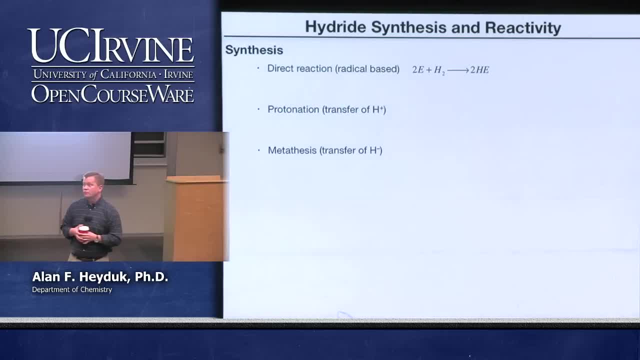 And nothing happens. And you wait for a really, really long time and nothing happens. And you heat it up. Guess what happens? Nothing. And then you take a strobe light and you flash it with the strobe light And then what do you think happens? 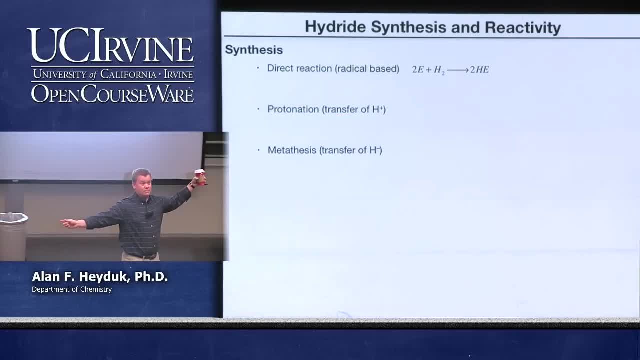 You blow the quarks out both ends and you make a big cloud of HCl gas. The reason: what happens there. you're like, oh, that sounds like a great demo. I want to snoop full of that in the morning. 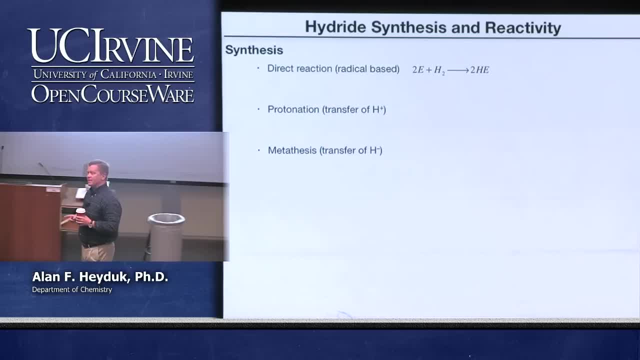 It'll wake you up, right, But what happens in that reaction is that chlorine, the chlorine Cl2, will absorb that flash of light And it homolytically cleaves the chlorine chlorine bond. You generate chlorine radical, which then reacts with the H2. to make HCl, And it's a self-propagated bond, And it creates a self-propagated bond. So that's what we're doing. We're going to do it the other way around, So that's what we're going to do. 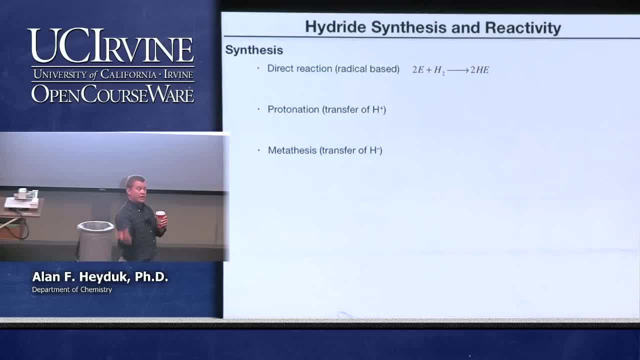 It's going to create a super-parameter And it creates a super-parameter reaction because then you spit out a hydrogen radical and it goes on. and it basically goes on until it consumes all of the hydrogen and all of the chlorine and it's very exothermic, as we saw on the last slide, so it heats up the gases. 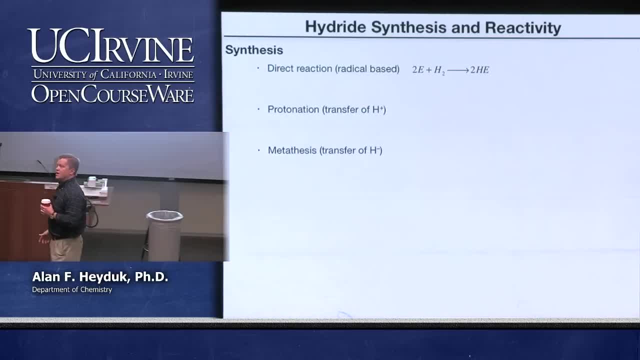 expand and they blow. I mean it's really, really a cool reaction because it just takes that one pulse of light and the whole reaction is over. that's all it takes to get over the activation barrier, and so that's the beauty of free radical reactions. the others, the ways of making hydrides, aren't that exciting. 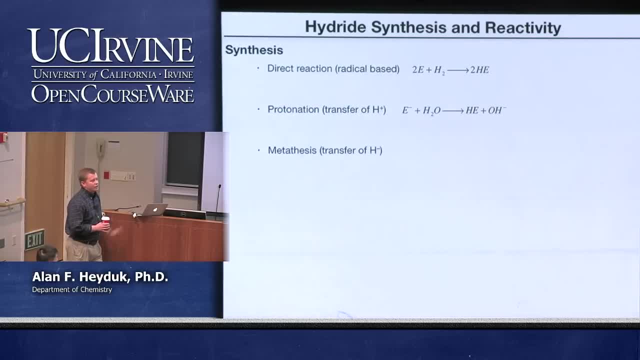 we can protonate stuff. okay, if we put, you know, the conjugate anion of some element into water, you can protonate it and make the the acid and hydroxide. or you can do a metathesis reaction: you take an element halide and react it. 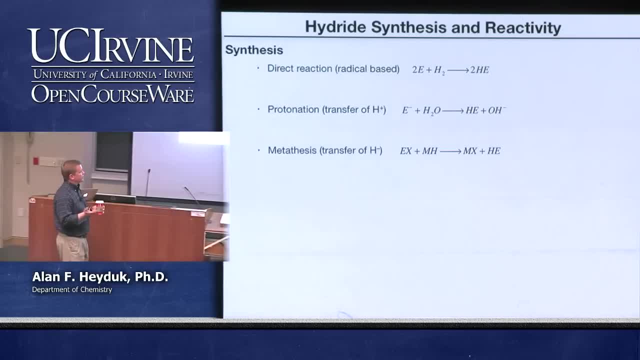 with a saline hydride, you get the metal. click you get the metal. halogen out the hydrogen at the acetate, you take one. you take a stainlessplaces, you stock the anion innovative, so you put yours in a said sure works to be a high, high. 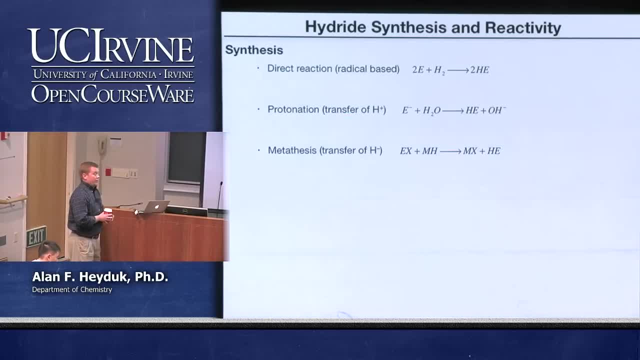 It's the salt and the corresponding hydride. And so now, when it comes to reactivity patterns, what do you know? it's the same three ways. So the first is that you can homolytically cleave. You can take that HE that you just formed. 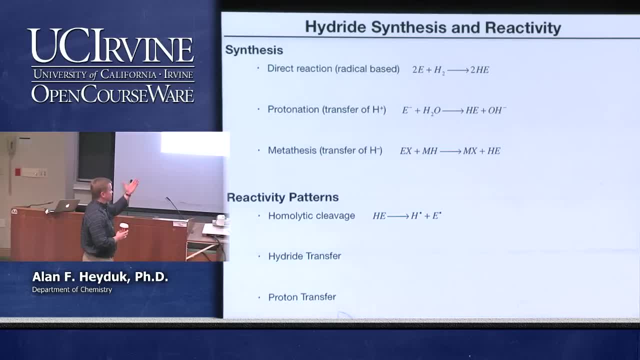 by a radical reaction and blow it back apart into H dot and E dot, You can transfer a hydride. The hydride transfer is just another way of talking about this metathesis reaction. Because if you think about that metathesis reaction, 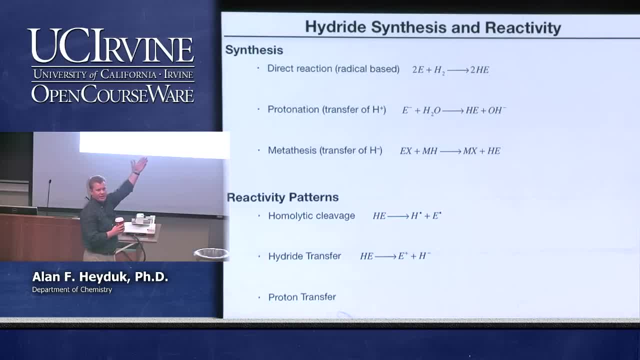 in a saline hydride it's M plus H minus. So what you're really doing is you're transferring a hydride H minus to the element E, And so same thing here. We're just reversing that process and splitting it. 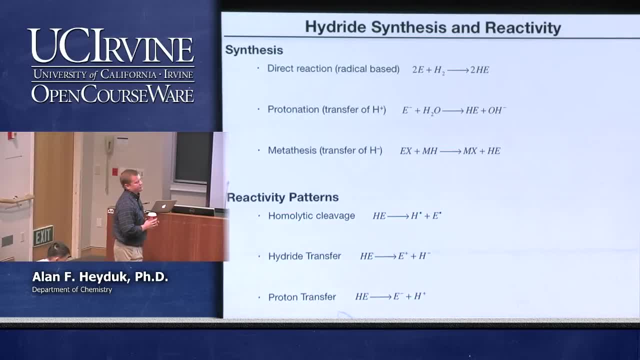 up as a hydride reaction And then, of course, proton transfer. So if we have HCl, it's probably going to react with H dot. It's going to react by transferring a proton, even though we often form it by the radical reaction. 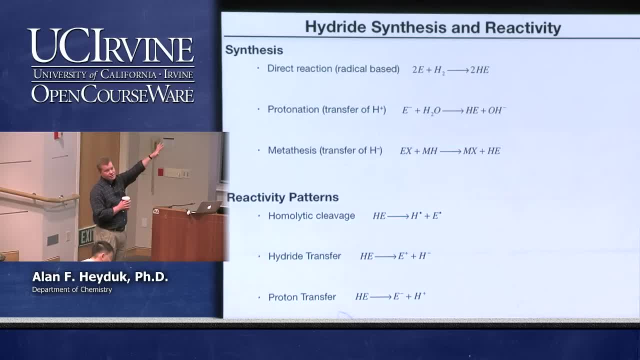 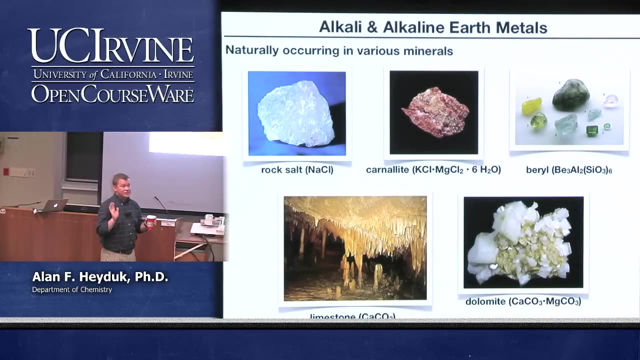 So just because you form a hydride by a radical reaction does not mean it has to react by that pathway, but it's going to be a pathway available. Okay, Enough about hydrogen. Ooh, pretty pictures. Yay, Alkali and alkaline earths. 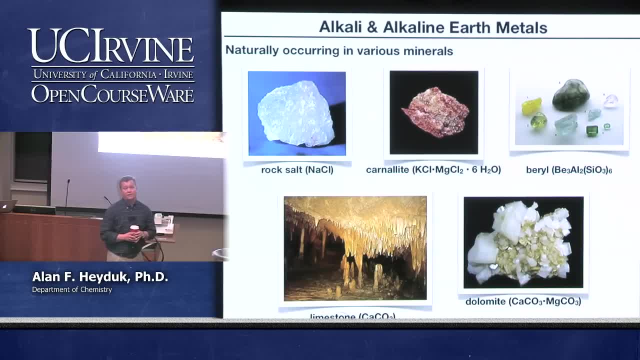 So these are the two things that we're going to be talking about. These are typically called, or often called, the rock-forming elements. Okay, So, rock salt, carnalite, beryl limestone. If you like to go spelunking, there you go. 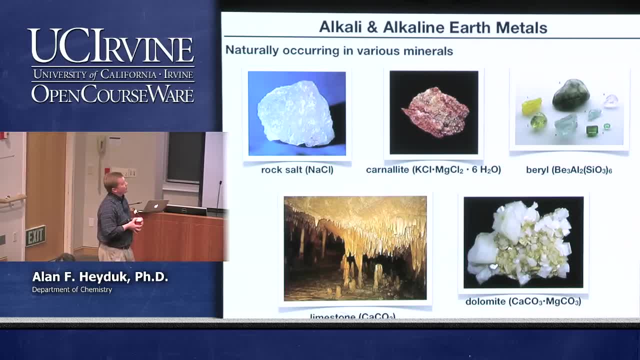 Dolomite. Anybody know what that real pretty square gem is in the beryl picture? An emerald? Yeah, That's an emerald. So these kind of complex crystals are, these are what give us our gemstones, And the gemstone color typically comes. 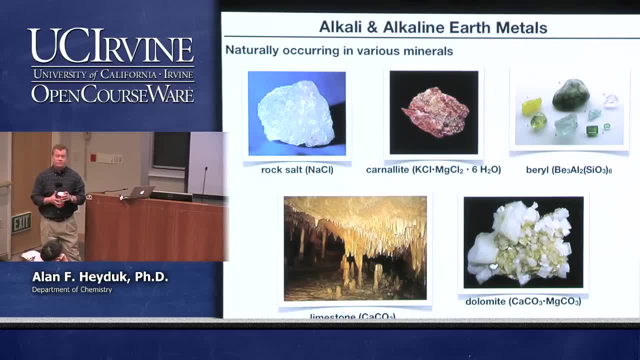 about from transition metal impurities in the structure. In this case, if you were to just have pure beryl, which is beryllium, aluminum and silicon and oxygen. it's that colorless one up in the right-hand corner. 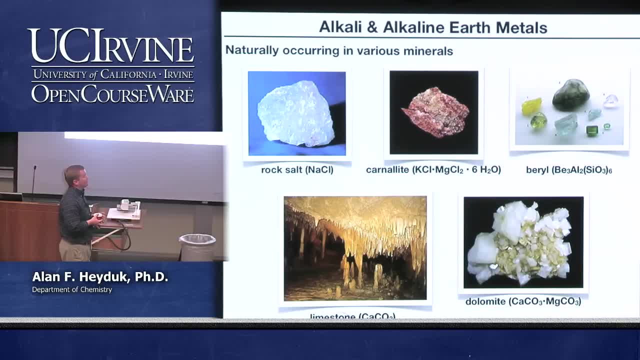 It's got no color. Those elements don't impart any color on the structure. But if you start introducing manganese or chromium or iron, impurities you can get. you can get various gemstones. Okay, We might. we probably will talk about that later in the quarter. 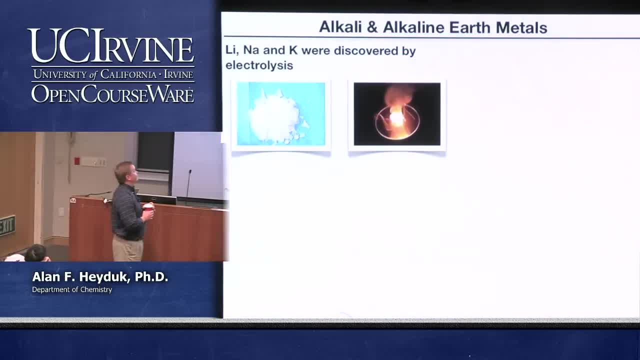 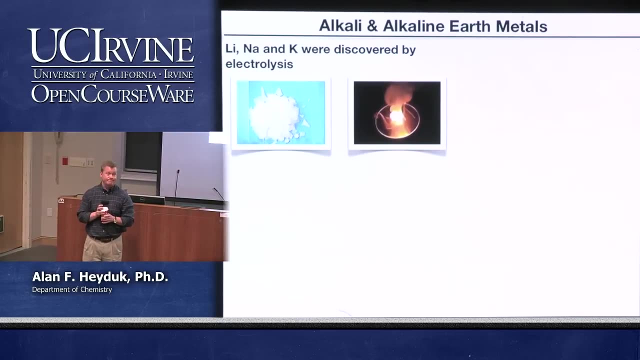 So how did we discover the alkaline and alkaline earth metals? Well, lithium, sodium and potassium were discovered by electrolysis. That's actually a scary thought to me. Has anybody seen what happens if you take sodium and you throw it in water? 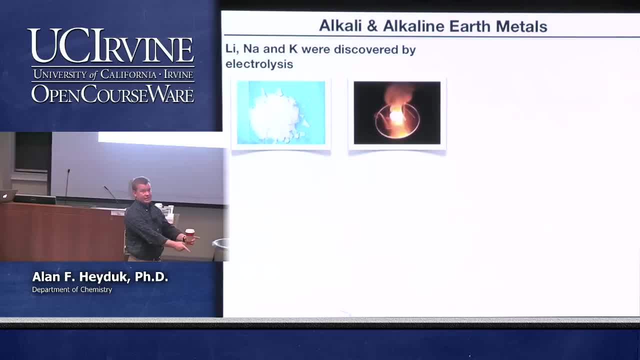 So in electrolysis what we do is we take a, we take a battery, we take two leads and we stick it in a salt solution and we just crank up the voltage until we start plating metal out. So you can imagine how spectacular that experiment was. 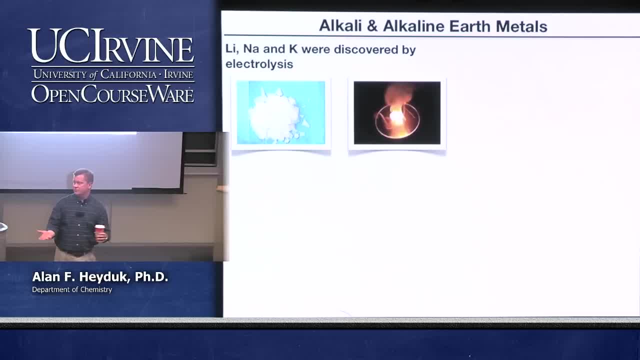 when somebody plated sodium out in the water solution. So another funny story. This is why we're never going to get through all this. So at MIT they used to do this great freshman chemistry demonstration to show how sodium reacts with water, And they would get a paint can. 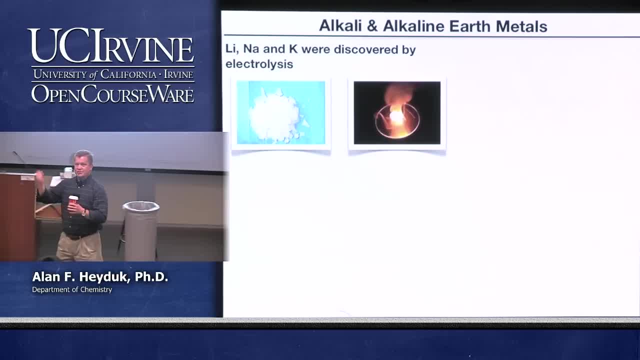 filled with sodium metal, take a screwdriver and jam holes in it, and then MIT is situated right on the Charles River, And so the whole freshman chemistry class of dorks would go out to the Harvard Bridge, stand there and the professor would be able to take the paint can. 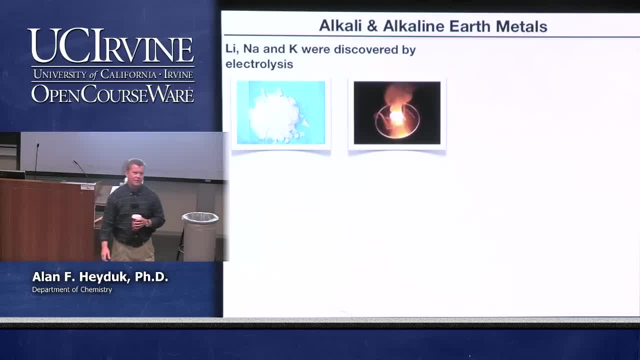 and close the paint can and throw it in the river. What happens is, of course, the water runs in through the holes and it sinks, and then of course, the water reacts with the sodium and makes hydrogen and comes up and hits the air. And there's a bunch of heat released and all of a sudden you get a big fireball, Burns off all the hydrogen starts filling with water, goes back down, fills with more water, more hydrogen is made, pops back up fireball. 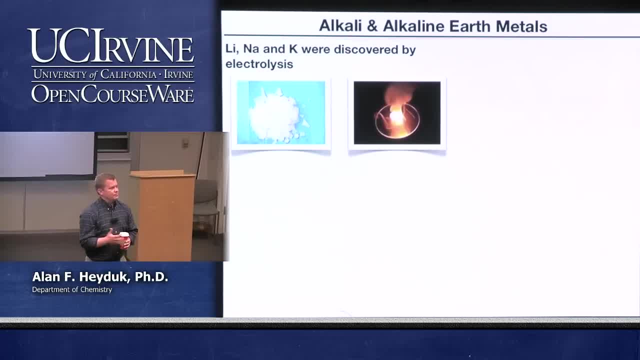 So here's the thing. They did this for years, and the problem is: as dorky as they are, the undergrads at MIT are also pretty smart, and somebody went through and did an acid-base calculation. Well, in addition to hydrogen, you're making sodium hydroxide. 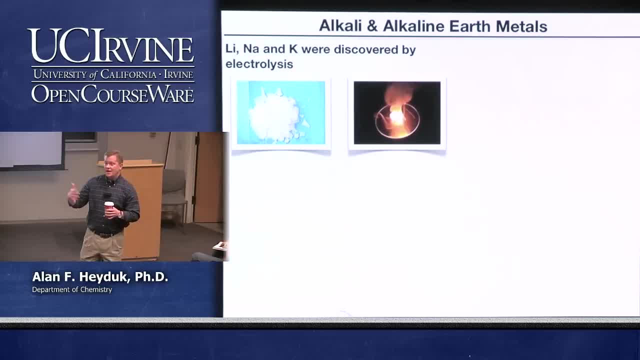 which is a strong. It's a very strong base and they calculated how much base they were making by this pound of sodium and they realized that it was actually changing the pH of the river and, you know, killing fish and stuff. okay. 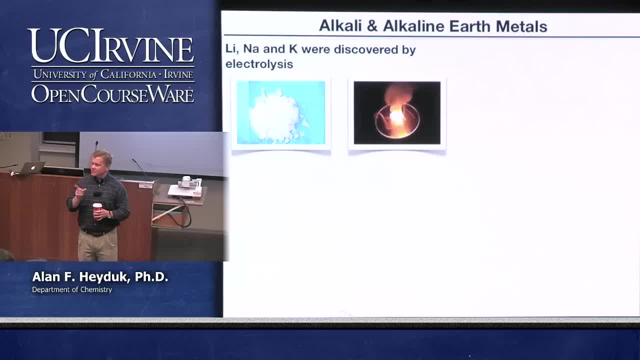 So with great power comes responsibility. okay, You can't just go throwing sodium metal by the pound into the river and the fish get very unhappy Anyways. So again, think about how much fun that electrolysis experiment was. Oh look, sodium. 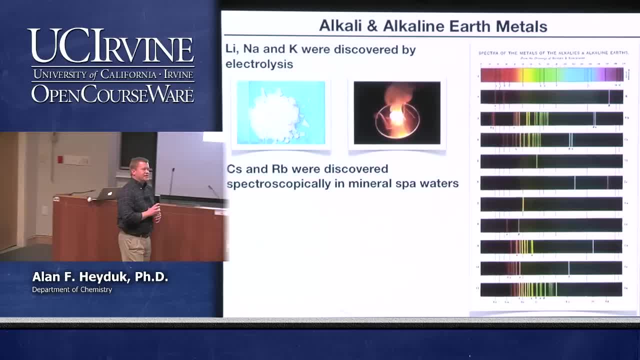 Pfft, Cesium and rubidium have a little bit less notable discoveries. so salt spas: we hear about these all the time. You know they make you younger and everything's wonderful. but you can do spectroscopy on these spas. 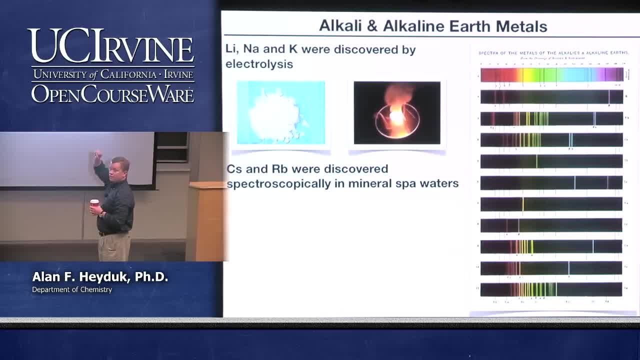 and we've seen these sort of Rydberg spectra where the ions give rise to lung And we can calculate the energy of the various orbitals from the spacing of these lines. We've done this probably in P-Chem And you can see rubidium is the third one there. 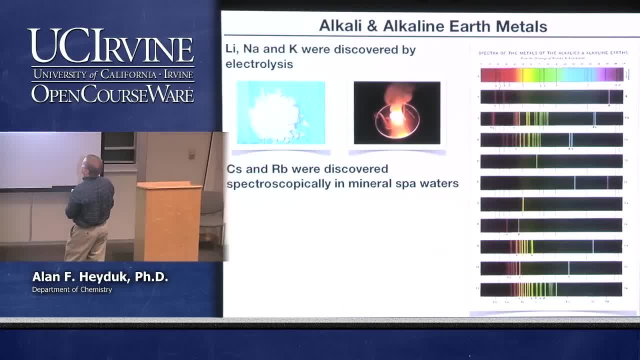 It's got a very pretty pattern. Let's see what was the other one. Cesium is- oh wait, oh- right below. rubidium also has a very pretty pattern, interestingly enough. So this is, they were discovered spectroscopically. 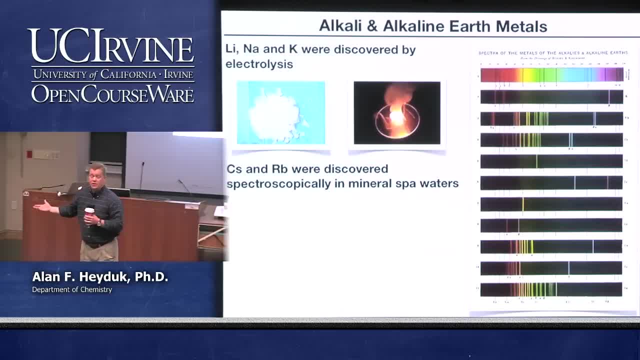 because they gave rise to lines for elements that we didn't know yet. But, interestingly, if you take these sort of alkali metal salts and grind them up really finely and wrap them up with some gunpowder and paper and set it off, well, that's how you make fireworks. 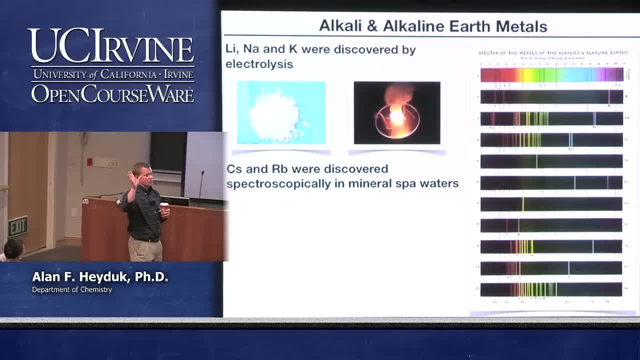 So potassium will give rise to a purple firework because, as it blows up, you're exciting these transitions and you can see potassium has that nice line out, the purple line that gives rise to it. All right, Let's take a look at the next one. 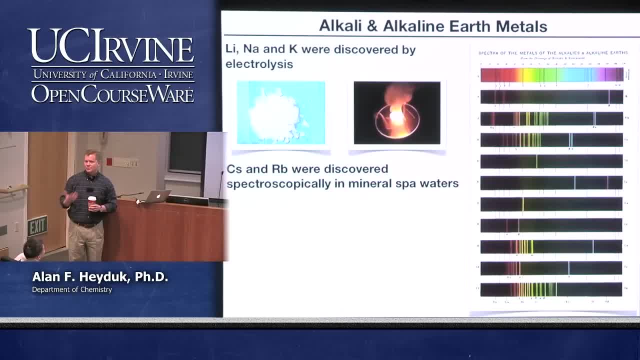 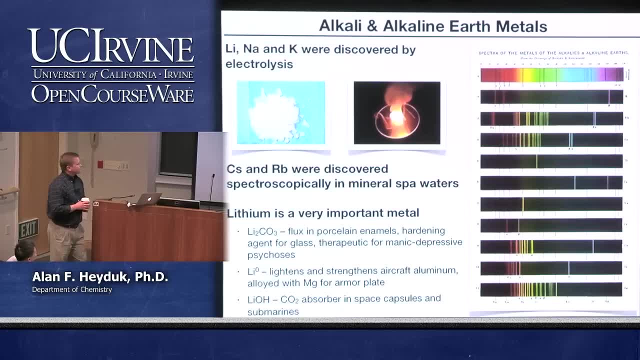 This one is called lithium carbonate. It's a very interesting one because it gives rise to the color. Have I mentioned that chemistry is really cool? You know how lucky you guys are to be chemistry majors. It's awesome. Okay, Lithium metal: very important industrially. 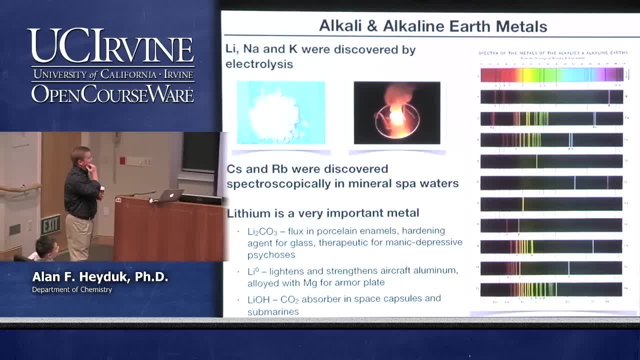 Lithium carbonate is a flux in porcelain enamels. Basically, it helps in their flow. It's a hardening agent for glass and, of course, a therapeutic for manic depressive orders. Lithium metal is used all the time. It's used all the time to alloy and lighten aluminum. 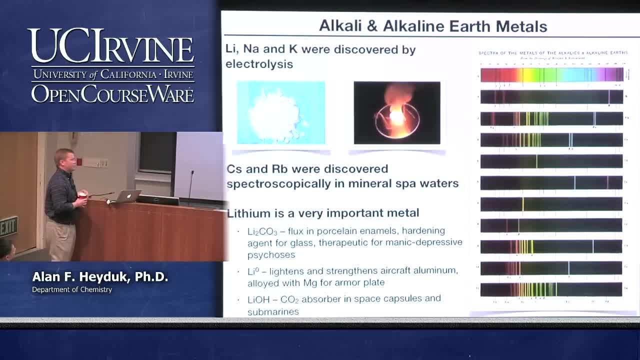 for things like planes. or you'll alloy it with magnesium to make armor plating. That's cool. I could use some armor plating Lithium hydroxide. that's the you ever wonder, like how they deal with carbon dioxide in the space station.